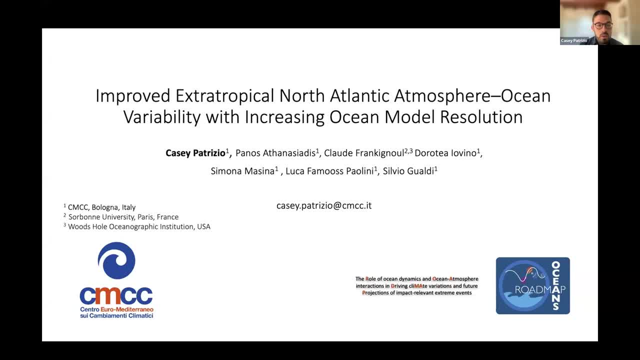 And this work was funded by a GPI Project called Roadmap, And I have to say I really enjoyed being a part of this project the first couple of years here at CMCC- Really great scientists- and I learned quite a lot. So, yeah, I hope you all find this webinar really useful, or at least somewhat useful, and please feel free to ask any questions at the end. 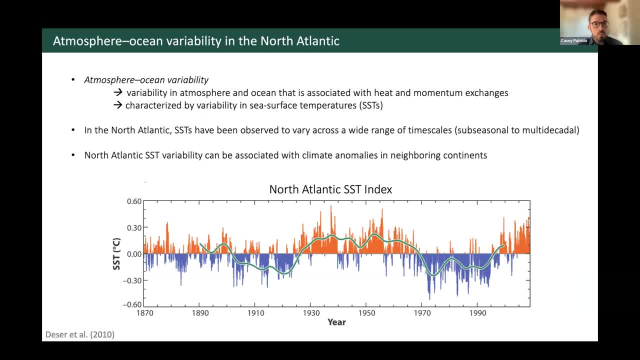 So, first of all, what do I do? What do I really mean by atmosphere-ocean variability? So, very broadly speaking, we can consider this to be either variability in the atmosphere or the ocean, which is associated with heat and momentum exchanges between the two media. 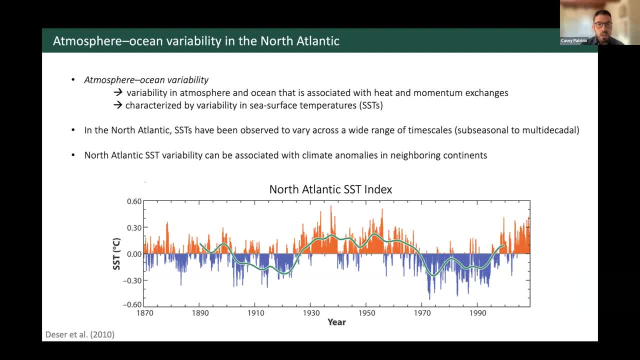 And so, because of this, it's generally characterized by variability in sea surface temperatures, That is, at the interface between the atmosphere and ocean. So, as you can see in this plot below, SSTs in the North Atlantic have been observed to vary across a wide range of time scales. 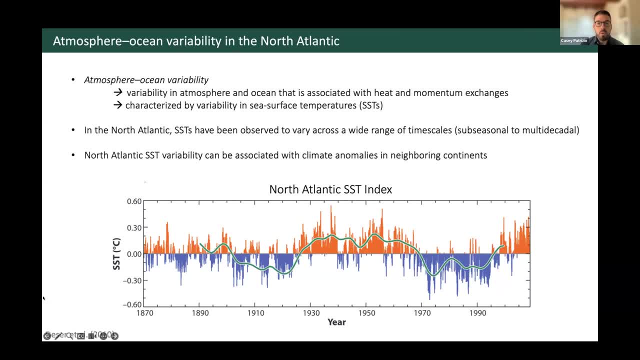 And so you can see some decades are cooler or warmer than others And, in general, as a scientific community, this is something we really care about, particularly because this variability tends to be associated with climate anomalies in neighboring continents, So, for example, precipitation and temperature anomalies over Europe or northern Africa. 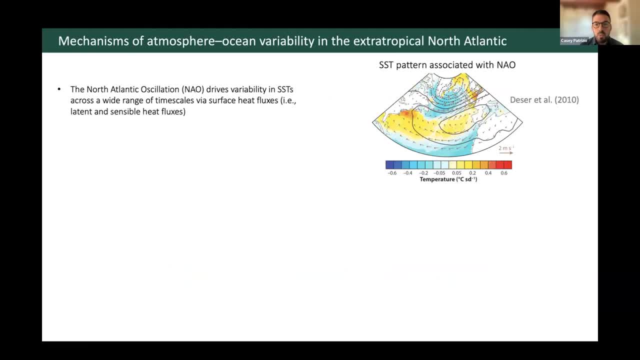 And so, focusing on the extratropical region, which is really the focus of our study, there have been a variety of mechanisms put forth for this variability, And so, if we start from the atmospheric perspective, it's very well known that the North Atlantic Oscillation drives surface heat flux anomalies which lead to sea surface temperature variability across a wide range of timescales. 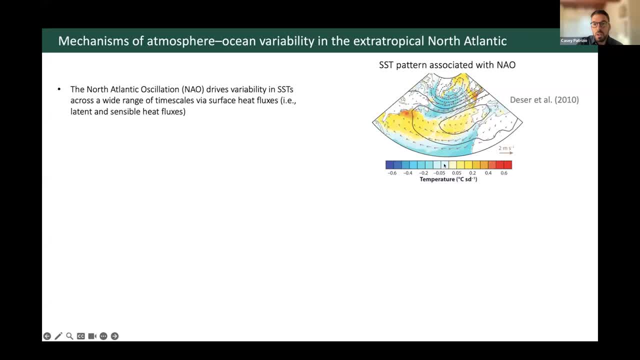 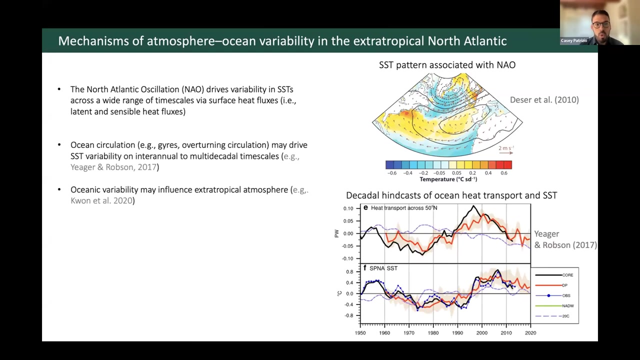 And with an SST pattern, looking something like what we see in this plot on the right. So this perspective of the atmospheric circulation driving oceanic variability Is really well established from many decades of research. But in recent years there's increasing evidence that the ocean circulation may play an important role for low frequency variability in this region. 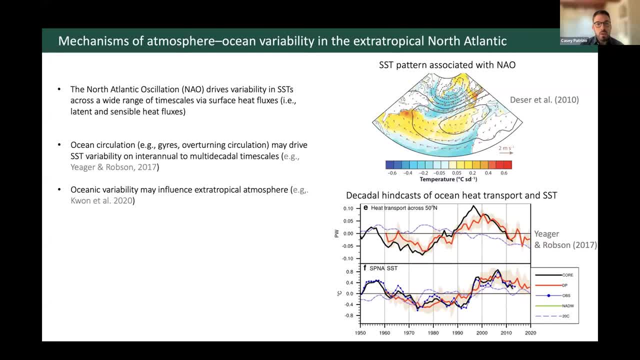 And so most of the evidence for this idea comes from modeling studies, And this is because we really don't have good observations of the ocean circulation, And so, as an example, here in the bottom right, I'm showing results from decadal hindcasts, which are just retrospective forecasts that have been initialized with ocean observations. 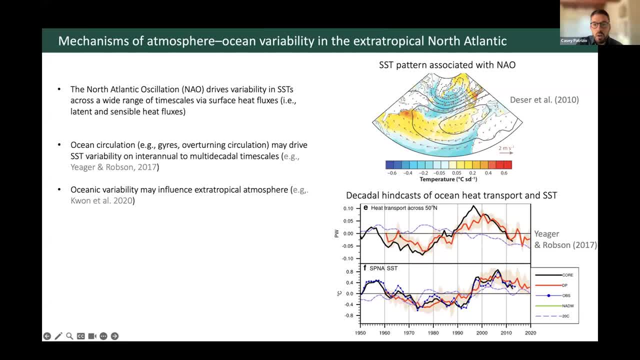 And so there you can see that variations in ocean heat transport across 50 degrees north are really quite consistent with SSTs in the subpolar North Atlantic region, And so this suggests that ocean circulation is playing an important role in this part of the North Atlantic. 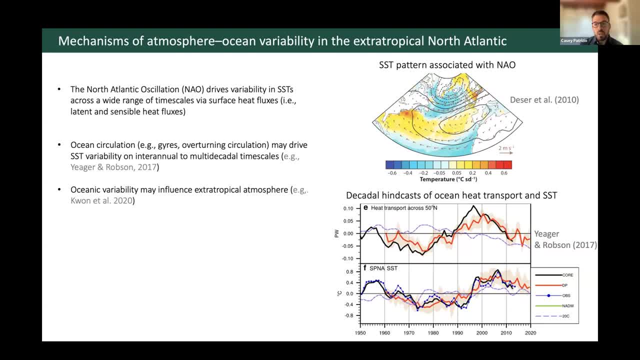 And so, even more recently, there's evidence suggesting that this oceanic variability can, in turn, influence the extra tropical atmosphere, And so this leads to two way interactions between the atmosphere and ocean. To complicate things even more, variations in external atmosphere variability can be very significant. 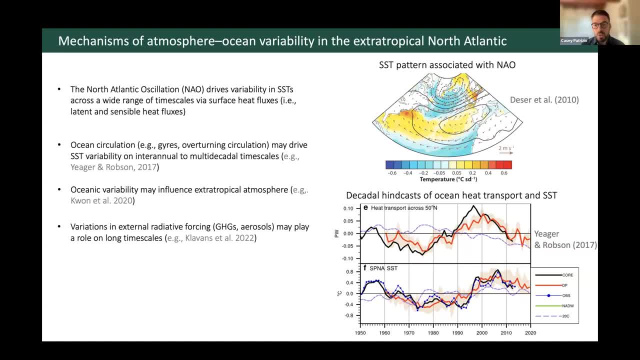 And external radioforcing, so, for example, associated with changes in greenhouse gases emissions or aerosols, have also been argued to play an important role in driving variability over the historical record, And so overall you can see a lot of processes potentially at play here. 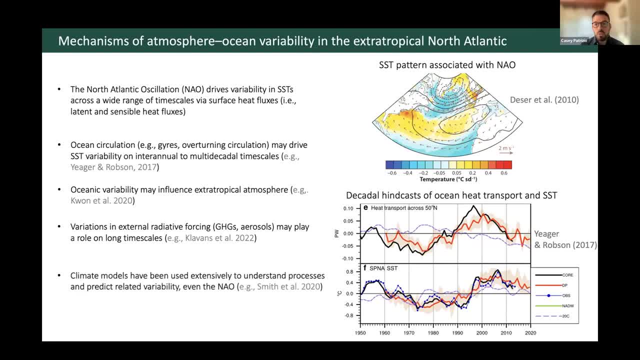 In general, climate models have been used to understand these processes But also predict associated climate changes, Climate anomalies. So, for example, recent studies have shown that even the NEO may be predictable on decadal time scales, And so I think this really motivates accurately representing these processes in climate models. 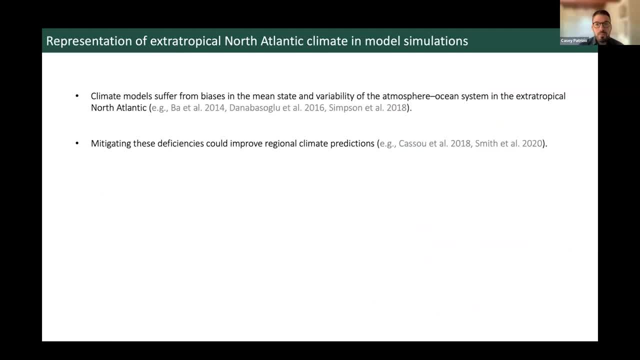 However, as we all know, climate models are far from perfect, And so they suffer from a variety of biases. involved the mean state and variability of the coupled atmosphere-ocean system in the extratropical North Atlantic region, And of course, this hinders the use of these climate models as tools for both understanding. 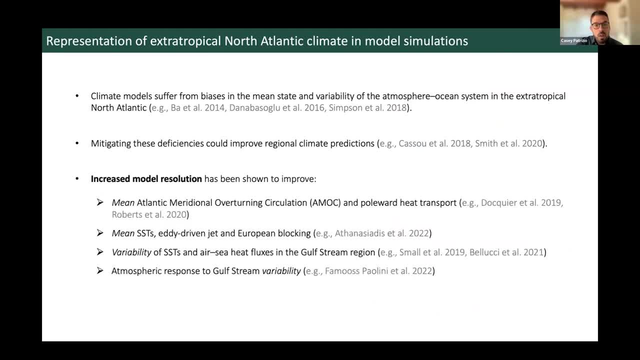 but also regional climate predictions, And so one way to mitigate these biases is through increased model resolution, And so, of course, resolution is not guaranteed to lead to a more realistic simulation, but there have been some studies showing some promising improvements in a variety of aspects. 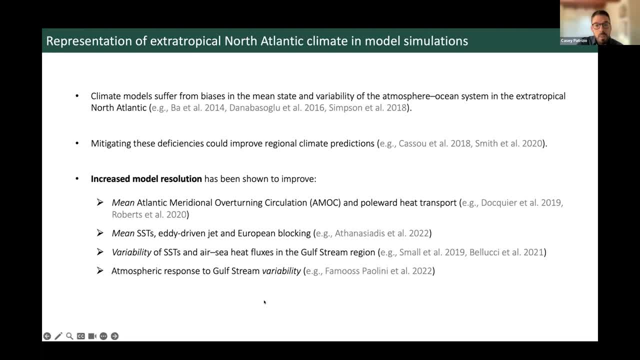 of climate in the extratropical North Atlantic region And so, for example, leading to improvements in mean SSTs, as well as Gulf Stream related variability, And so, of course, resolution is not guaranteed to lead to a more realistic simulation, but there have been some studies showing some promising improvements in a variety of aspects of climate in the extratropical North Atlantic region, And so, of course, resolution is not guaranteed to lead to a more realistic simulation, but there have been some studies showing some promising improvements in a variety of aspects. 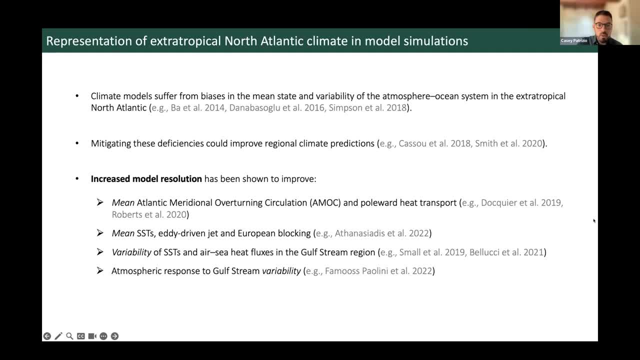 of climate in the extratropical North Atlantic region. So I won't say too much more about these improvements because in a few moments I'm actually going to highlight some of these studies. So I won't say too much more about these improvements because in a few moments I'm actually going 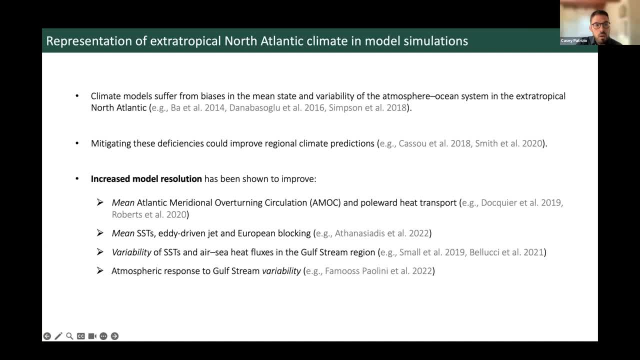 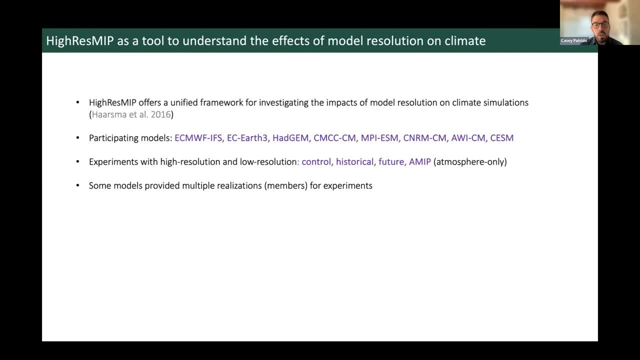 to highlight some of these studies. For now, I just want to introduce you to HiresMIP, which is a multi-model inter-comparison project that we've used in our study and many others have used to investigate the effects that model resolution has on simulated climate. 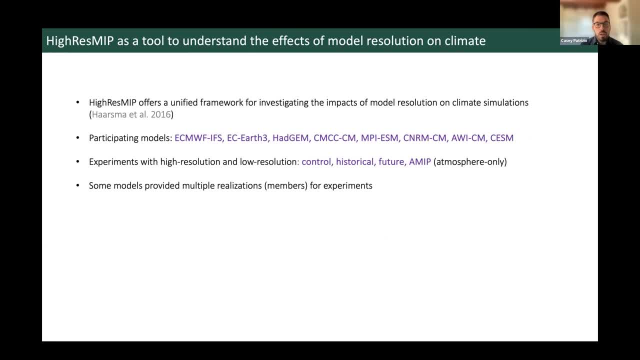 And so, as you can see, a number of modeling institutions are mostly using these technologies. institutions have participated in this and each provide a variety of experiments run on both high resolution and low resolution model configurations. So, in particular, they provide a control run. so that's with fixed radiative forcings, a historical run, which is with time-varying. 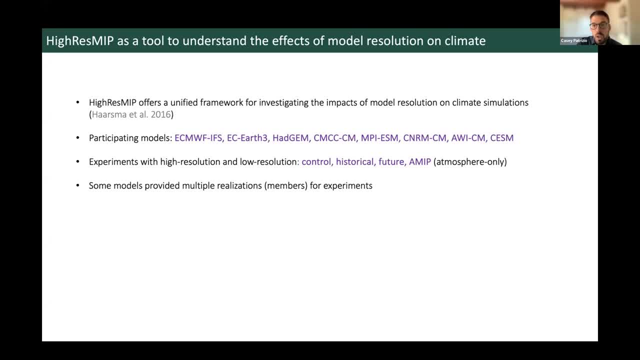 observed radiative forcings, future scenarios and AMIP runs. Those are atmosphere only with prescribed SSTs, And so one useful aspect of high-res MIP is that some of the institutions provided multiple members for some of these experiments, and this is particularly useful for 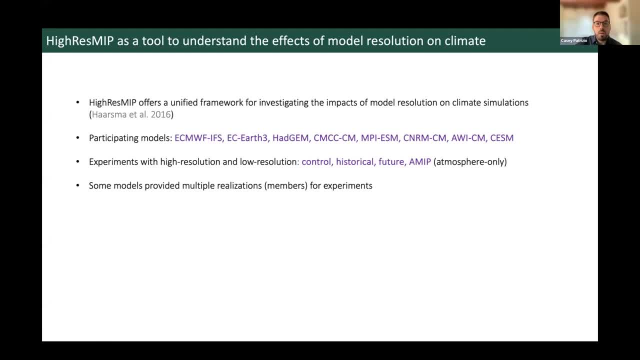 identifying some of the more robust effects of model resolution: High-res MIP. very useful, but not without shortcomings. So one of those is that the majority of the models use the same ocean model, NEEMO, And so I think this is being. 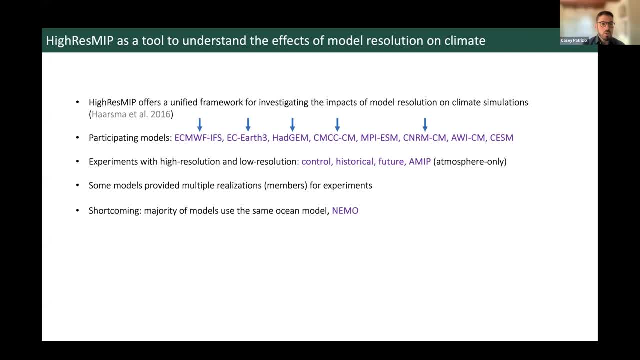 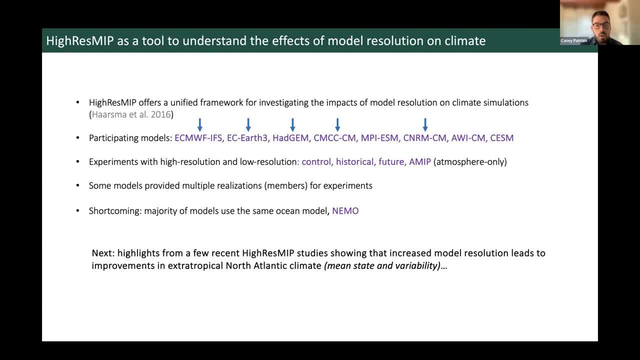 climates that arise from increased model resolution, And I'll focus on studies that use high-res MIP. So first I'll discuss mean states and then I'll move to variability. But hopefully by the end of this webinar you'll see that these two aspects are really quite. 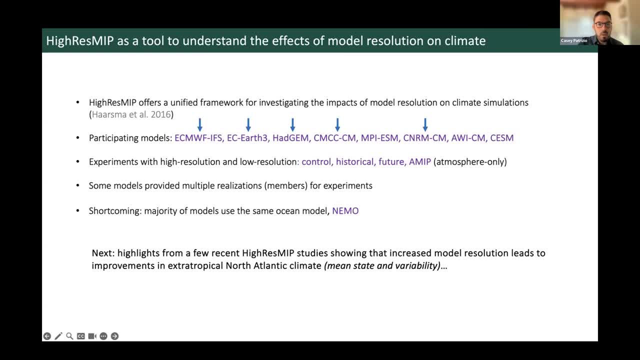 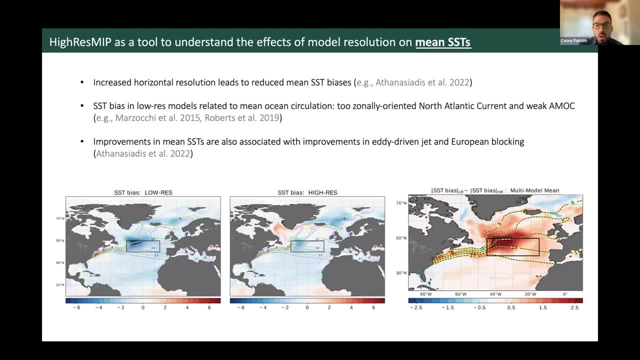 related in this region. Okay, so the first study that I'll highlight is from Athanasiatis et al, 2022.. Showing that increased horizontal resolution leads to large improvements in the mean SST field, particularly in the extra-tropical North Atlantic, which you can see below. 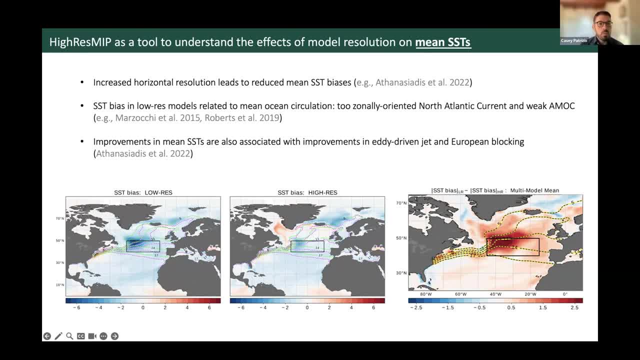 So, looking there, you'll see that the low-res models suffer from this cold SST bias at the end of the North Atlantic current, otherwise known as the Gulf Stream extension, And previous studies have shown that this is related to the mean ocean circulation. So in particular, LR models tend to have two zonally-oriented North Atlantic current and 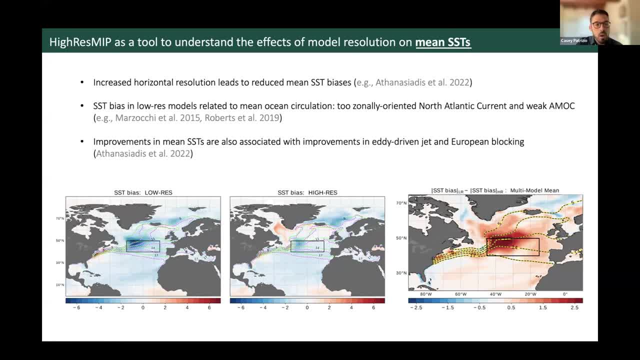 relatedly, a weak AMOC, and so this leads to less heat transport into this region. These deficiencies generally improve as we increase the level of heat transfer. Okay, the model resolution. thanks to resolving smaller scales in the ocean, particularly fine scale bottom topography, which is really important for shaping the ocean circulation in this. 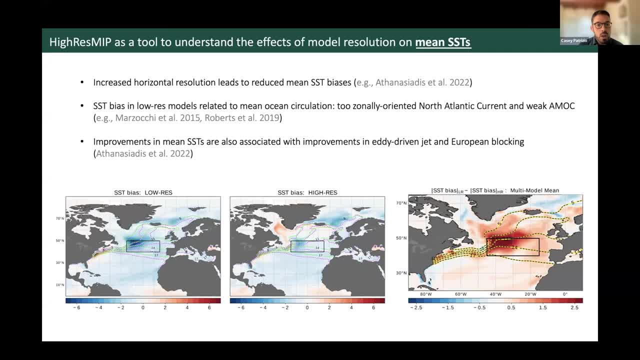 region. So in this study they also showed that these improvements in SSTs are associated with improvements in the eddy driven jet and European blocking. So just to say that model resolution also leads to other important climate impacts, not just in the ocean. 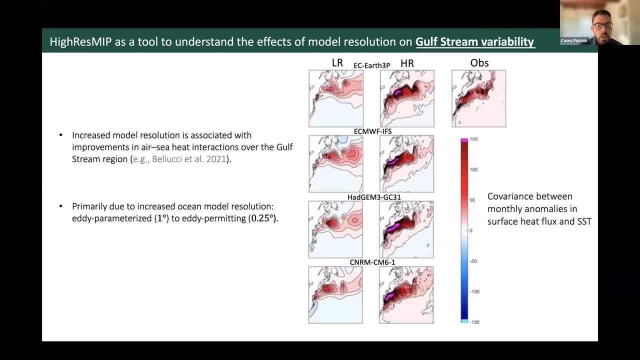 Okay. so coming to the variability, many studies have shown that- sorry about this, just hide this- whoops. Okay. Many studies have shown that model resolution is really important for accurate representation of air-sea interactions over the Gulf Stream region, And this is supported by Bellucci. 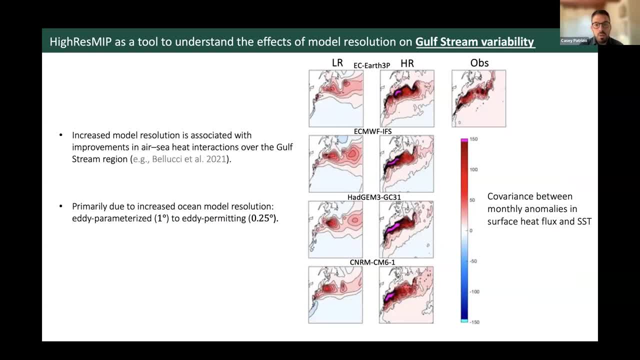 et al's analyses of high-res MIP simulations, And so this is what I'll highlight here. So in these plots you can see the covariance between surface heat flux and SST anomalies- Okay For observations- as well as a variety of models from high res MIP. 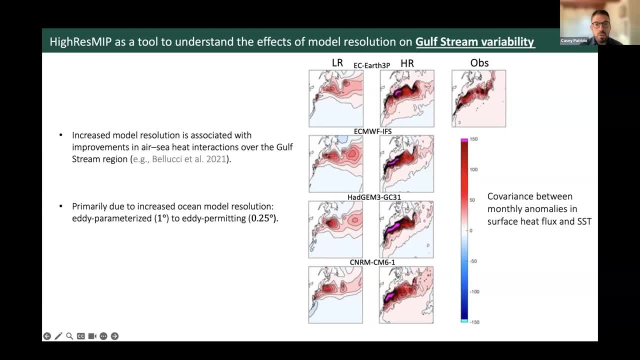 In all cases you see this positive covariance, which is indicative of the Gulf Stream related variability driving heat fluxes into the atmosphere. However, the HRI models have a much more realistic pattern. So if you look at the LR models, you can see that the covariance. 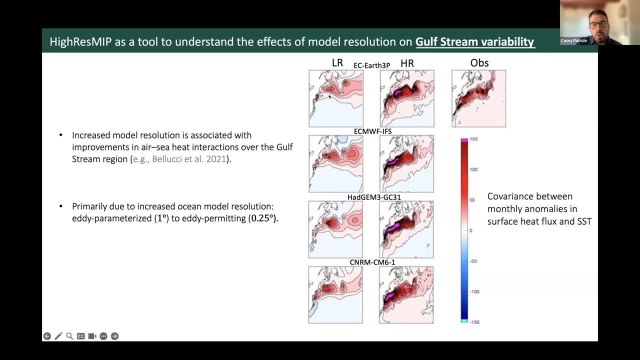 is quite a bit weaker, occurred in the plates, but thenGSコ人에서נם 되면 생성innen nella airule. And there's the indication that the Gulf Stream extension is too zonally oriented, as I mentioned before, And so in this study they show that this is primarily due to increased ocean model resolution as we move from eddy parametrized to eddy permitting. 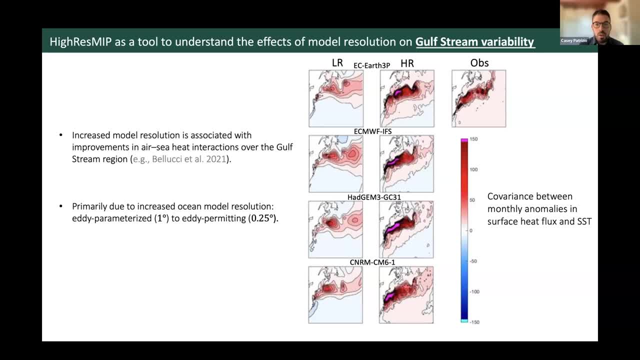 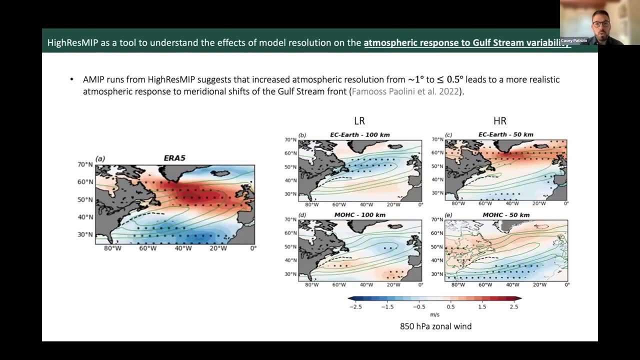 And so this just emphasizes the importance of resolving the ocean mesoscale in air-sea interactions over the Gulf Stream region. Okay so, finally, I just wanted to highlight some results from a recent PhD graduate of CMCC. Luca Fumus Polini did some really nice analysis of the AMIP. runs from HIRA's MIP. 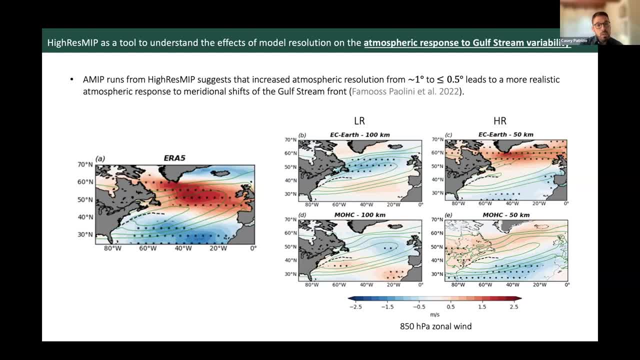 And basically showed that the atmospheric response to meridional shifts of the Gulf Stream front become more realistic as the atmosphere changes, And so, in particular, as you can see in these plots, there is a northward shift of the eddy-driven jet in association with a northward shift of the Gulf Stream front, which is really only present in the HR simulations. 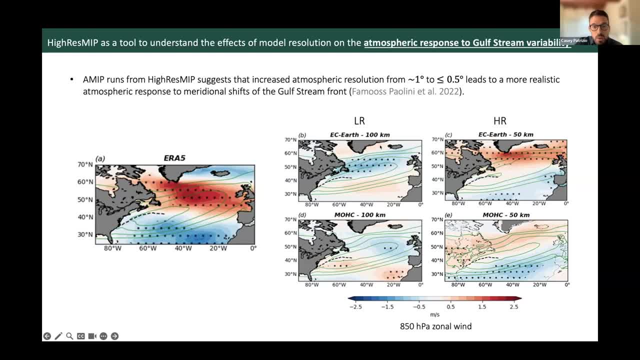 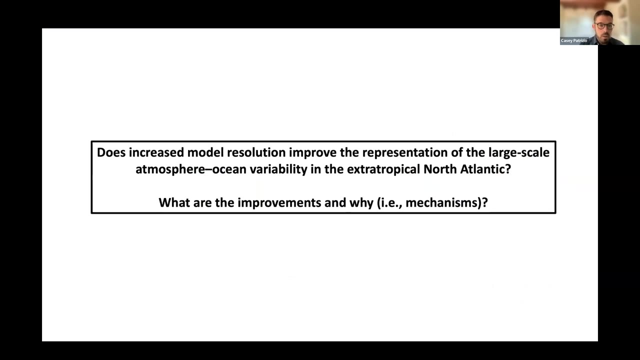 And the LR simulations apparently failed to capture this relationship, And so this is a really interesting study. And so this is a really interesting study, And so this suggests that atmospheric resolution may also play an important role in atmospheric ocean variability in this region. Okay, so, very broadly speaking, I think we know from previous studies that ocean or model resolution is really quite important for Gulf Stream related variability. 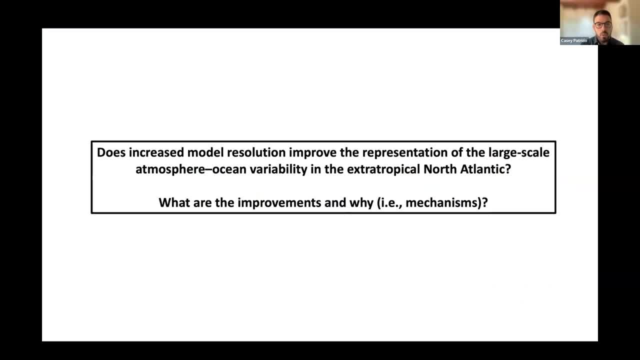 But it still remains somewhat unclear whether increasing the model resolution leads to robust improvements in the ocean. So I'm curious as to whether and where the effectiveness of the good pilot study is more strain probably in the atmosphere için variability when we consider the broader extra-tropical North Atlantic region. 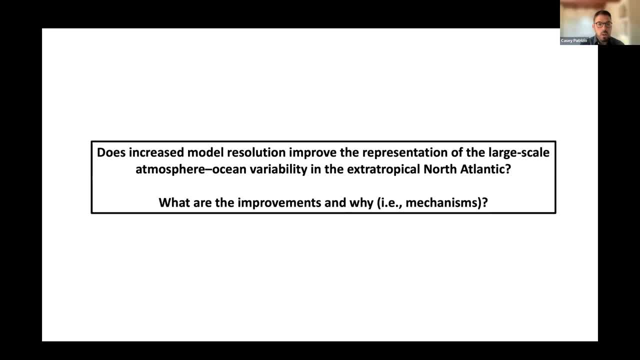 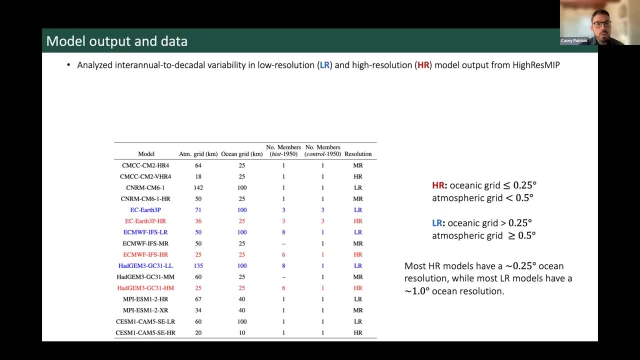 So this is the question we're addressing in our study, focusing on whether there are improvements and what the specific mechanisms are. And so we addressed this question through analysis of the interannual to decadal variability of both low-resolution and high-resolution models from the high res MIP, And I'm showing those models here in this table. And so, since the 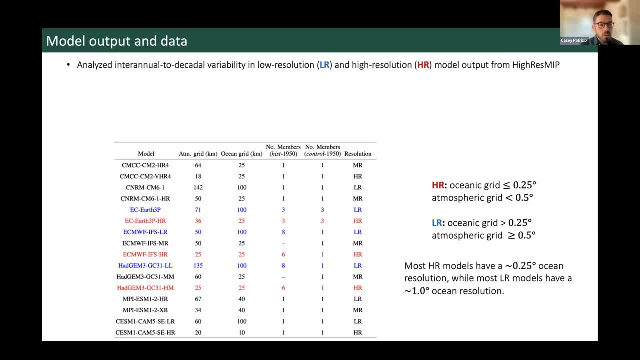 specific resolutions vary between modeling institutions. we came up with our own definition of HR and LR. You can see on the right here. In general, most of the HR models have a quarter degree ocean resolution, while most of the LR models have a one degree ocean resolution. 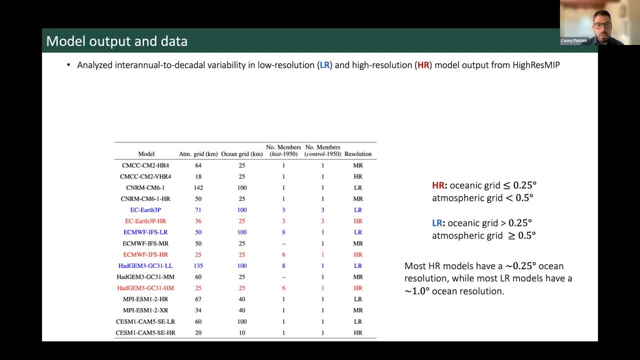 Whereas the atmospheric resolution cutoff is a half a degree and is a bit more variable, in general, between the different models. So then, we analyzed sea level pressure and different oceanic variables from the historical and control simulations, Focusing primarily on the models with multiple members in the historical runs. 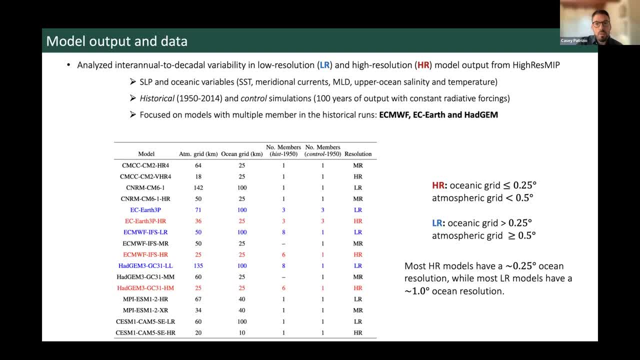 So that's ECMWF, ESEARTH and the HADGEN model, which I've highlighted here in blue and red. Finally, then, comparing, we compared these simulations to ERA5 atmospheric reanalysis, as well as observations from EN4 between 1990 and 2000.. 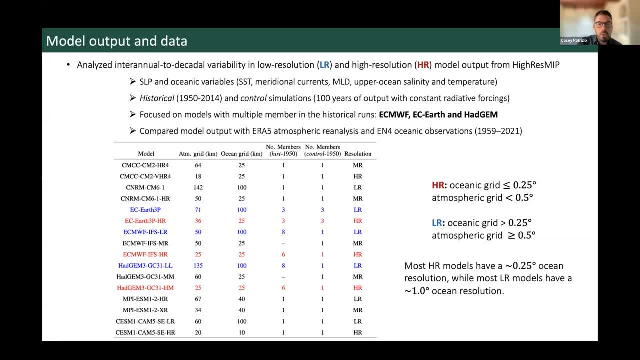 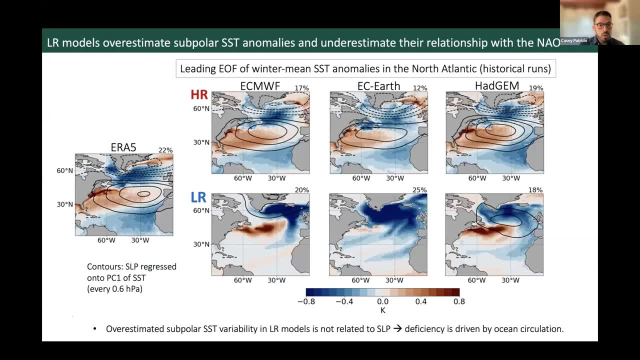 And we also compared these simulations to ERA5 atmospheric reanalysis from EN4 between 1959 and 2021.. Okay, coming to some results now. Just to start things off here, I'm showing the leading EOF of winter mean SST anomalies in the North Atlantic and the associated sea level pressure anomalies. 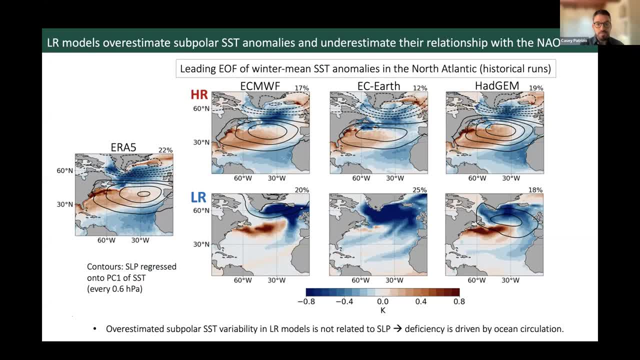 And these results are for the historical runs, And so you can see immediately that the HR models shown in the top row do a much better job of capturing the tripole SST pattern and associated NEO-like sea level pressure that we see in ERA 5.. reanalysis shown on the left. 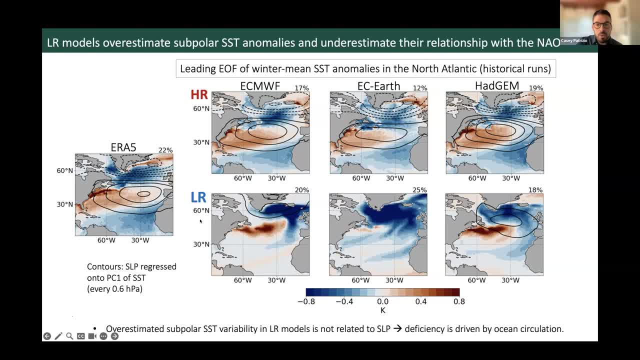 Surprisingly, the LR models fail to capture this very fundamental pattern. So, in particular, they overestimate SST anomalies in the subpolar region and severely underestimate their relationship or their correlation with the NAO. And in fact, if you look at the LR simulations, 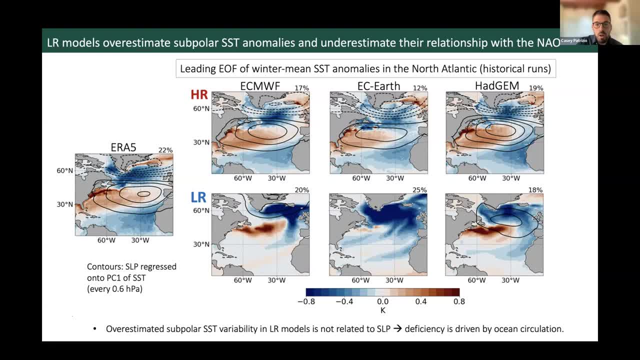 there really aren't any coherent sea level pressure anomalies associated with this SST variability, And so this suggests that this deficiency is driven by the ocean circulation. So we can try to understand the timescale dependency of this SST deficiency a little bit better, And to do this we average SST anomalies over this yellow box. 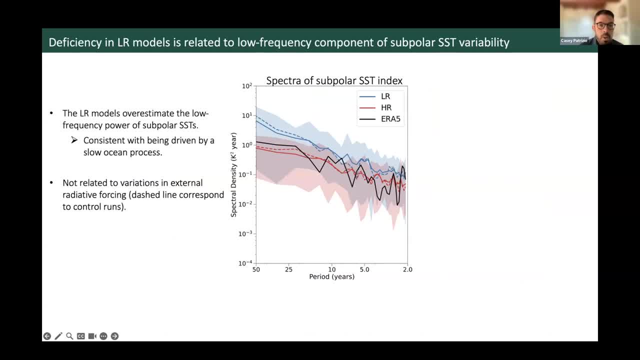 and calculate the spectra, and that's shown here, And so, as you can see, the LR models tend to have much more power on low-frequency timescales compared to the HR models and 8-ERA-5 reanalysis, And so this suggests that this deficiency we're seeing 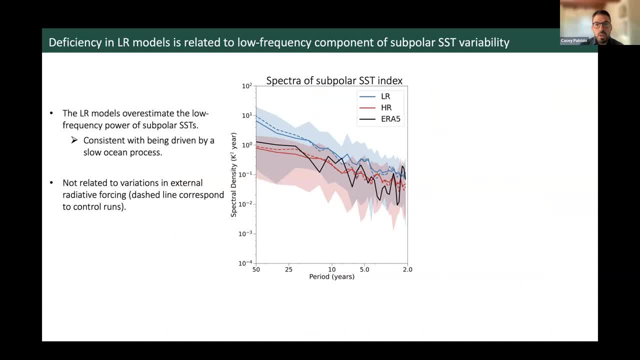 is related to the low-frequency component of the SST variability, which is consistent with being driven by a slow ocean process. So we also found that this is not related to variations in external radiative forcing. So the results for the control runs are shown as the dashed lines here. 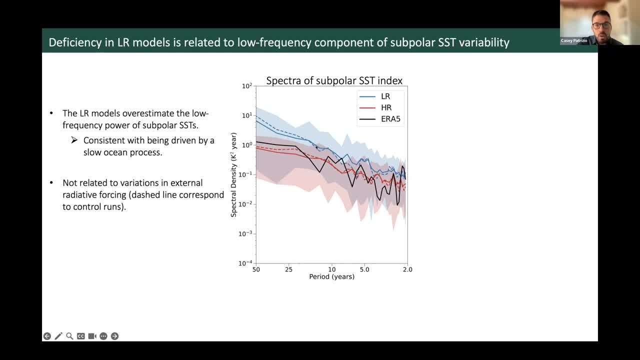 And you can see they're really quite similar to the solid lines which are the results, And you can see they're really quite similar to the historical runs. Finally, we also found that this is not related to differences in the spectra of the NAO itself. 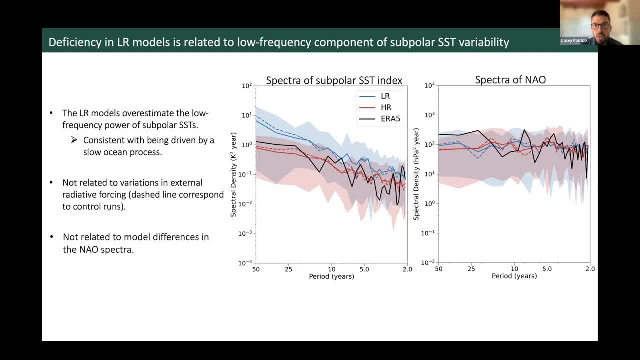 So you can see on the right, really quite similar between HR and LR models, And so everything here is pointing to something going on with the ocean circulation. So for the rest of the webinar, I'm basically going to focus on a few things. 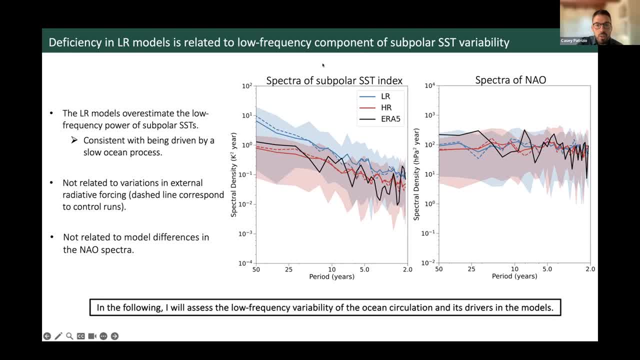 So I'm going to focus on a few things. So I'm going to focus on a few things. So I'm going to focus on explaining what's driving these differences between the HR and LR models, focusing on the low-frequency variability of the ocean circulation and its drivers. 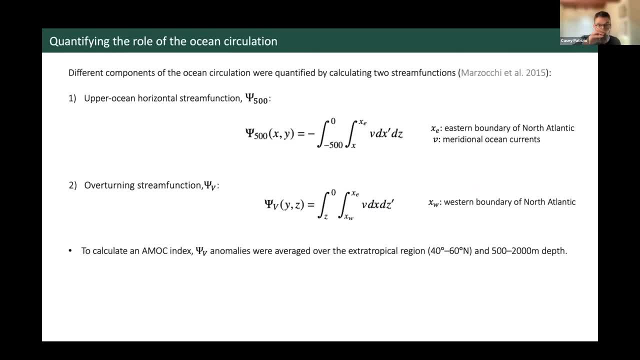 Just get a glass of water, Okay, So, in order to quantify the role of the ocean circulation, we followed a method from Marzocchi et al's 2015 paper. So, in order to quantify the role of the ocean circulation and its drivers, 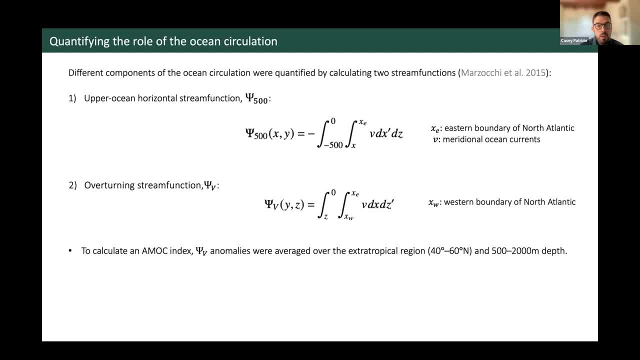 we followed a method from Marzocchi et al's 2015 paper and calculated two different stream functions from the meridional ocean currents. So I'm showing the formula here just for reference. Basically, we calculated an upper ocean horizontal stream function. 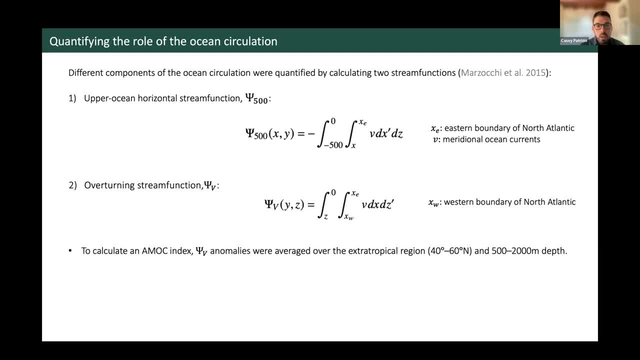 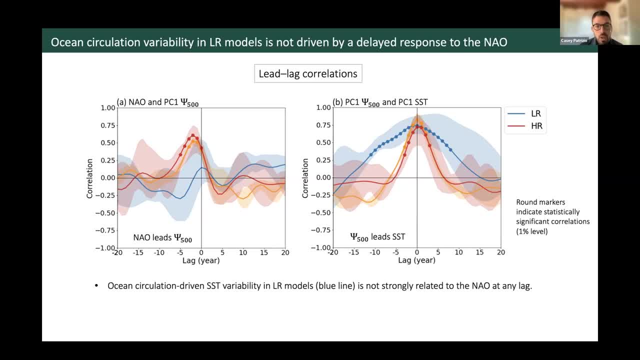 This was in order to quantify variability in the upper ocean horizontal system. This was in order to quantify variability in the upper ocean horizontal system stream function, And so this suggests that the atmosphere is not driving this variability, this ocean variability that we're seeing, And so it's likely to be coming from a process. 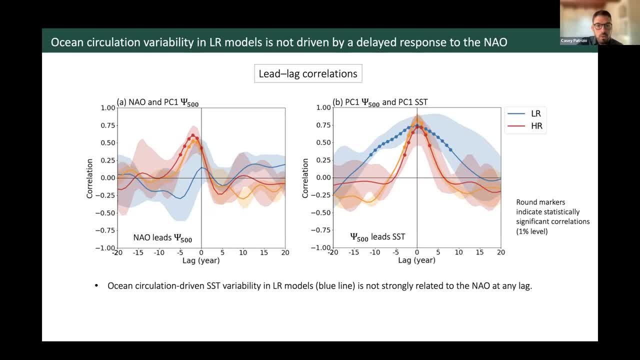 that's intrinsic to the ocean And that's what I'll show a little bit later. So this is really quite in contrast to what we see in the HR models, where there's a much stronger relationship with the NAO, indicated by the red lines here. 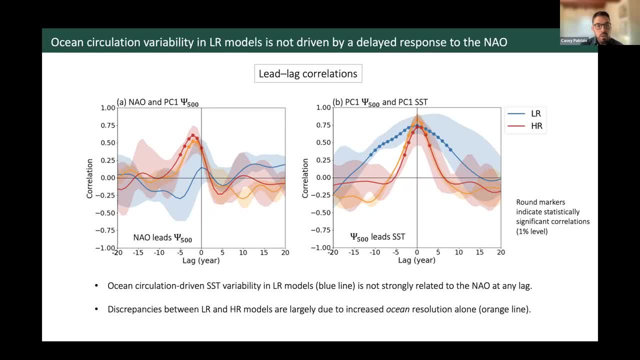 So we also analyzed a subset of simulations in which only the ocean resolution was increased, And those results are shown by the orange line in these plots. And so in this case you see a large agreement with the HR simulations in which both ocean and atmospheric resolution was increased. So this suggests that 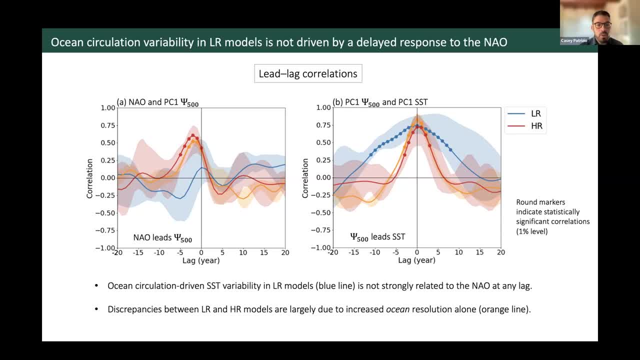 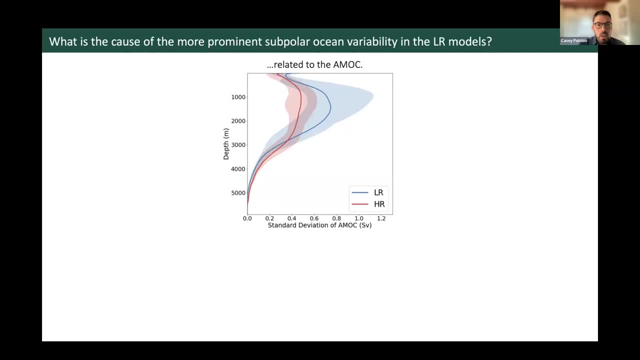 the ocean resolution was increased, And so this suggests that the ocean resolution was increased. Ocean resolution is really responsible for the differences between the HR and LR simulations and emphasizing again the importance of ocean processes. Okay, so the next thing that we explored was the role of the AMOC. 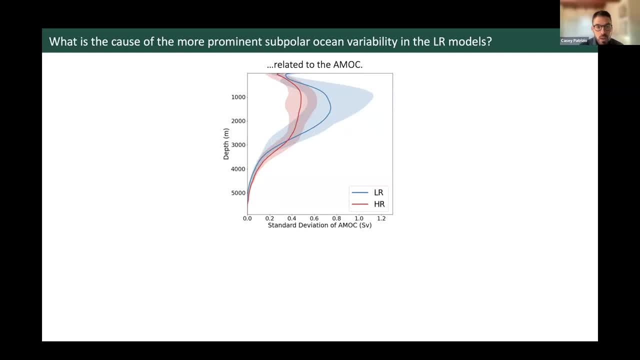 This is motivated by previous studies showing that subpolar variability is tends to be associated with AMOC variations, And so it turns out the AMOC is really key to understanding the differences between the models, And so this is motivated here. in terms of the 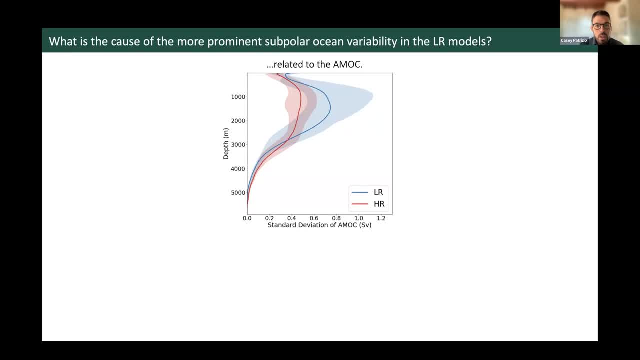 standard deviation of the AMOC, which clearly indicates that the LR models have much greater low frequency variance compared to the HR models. And so now for the rest of the webinar, I'm going to transition to explaining what the AMOC is. And so I'm going to start by explaining what the 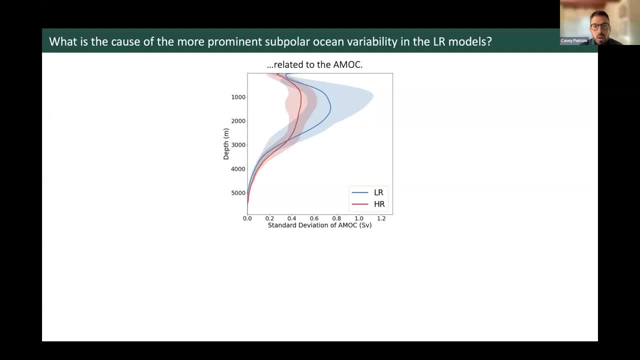 AMOC is, And so I'm going to start by explaining what the AMOC is, And so I'm going to start by explaining what you're driving this larger variance of the AMOC in the LR models. And so, since there are a few different steps to these, to this explanation I thought I'd give you. 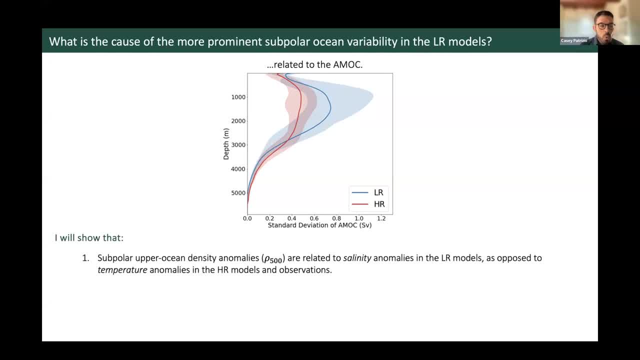 a brief preview of what's to come. Don't worry if it doesn't make sense now. hopefully everything will be more clear at the end. So first we analyze subpolar upper ocean density anomalies, which are an important driver of the AMOC, And then we analyze subpolar upper ocean density anomalies. 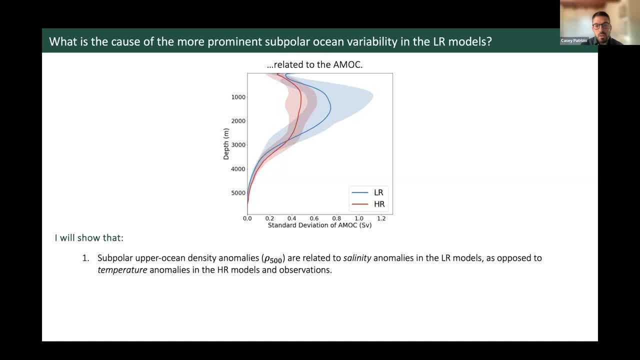 which are an important driver of the AMOC. And then we analyze subpolar upper ocean density anomalies, which are an important driver of the AMOC. And then we analyze subpolar upper ocean density anomalies and we found that these density anomalies tend to be related to salinity. 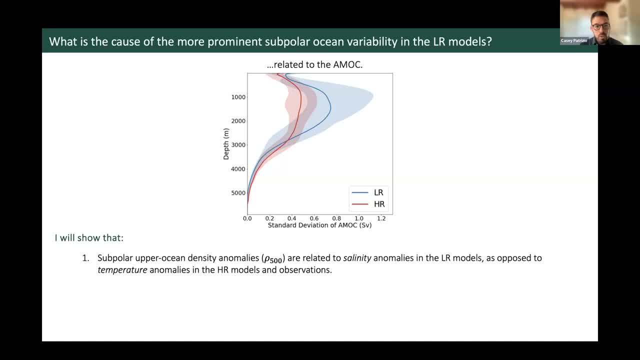 in the LR models, while they tend to be related to temperature in HR models and observations. Next, we explain this in terms of differences in the upper ocean mean state of a key deconvection site. So show that that there's a colder, fresher mean state in the LR models, which then favors a salinity conversion. 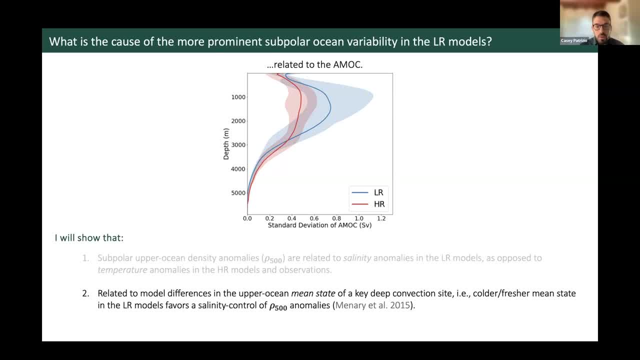 Next, we explain this in terms of differences in the upper ocean mean state of a key deconvection site, control of density anomalies in this region, And then, finally, I'll argue that this ultimately promotes the greater low-frequency variance of the AMOC, as well as different subpolar. 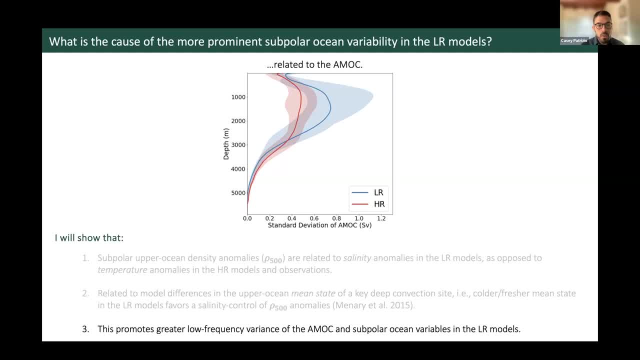 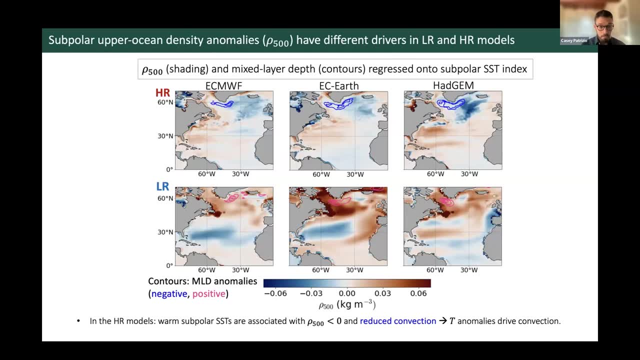 ocean variables that we see in the LR model runs. Okay, so first coming to the upper ocean density. So here I'm showing upper ocean density anomalies as well as mixed layer depth anomalies as a proxy for oceanic deep convection. both regressed onto a subpolar SST index. 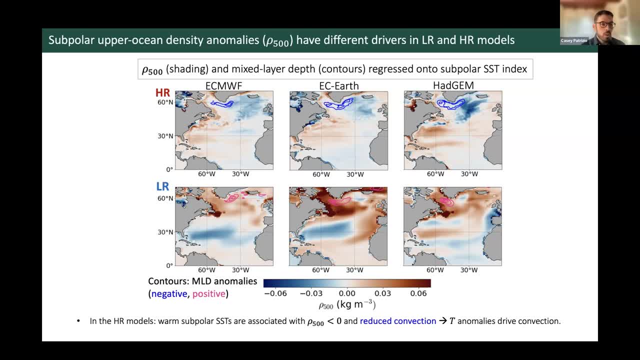 So this really gives us a sense of the upper ocean density anomalies and convection anomalies that tend to be associated with a warm SST anomaly in the subpolar region. So if we focus on the upper ocean density anomalies, we can see that the upper ocean 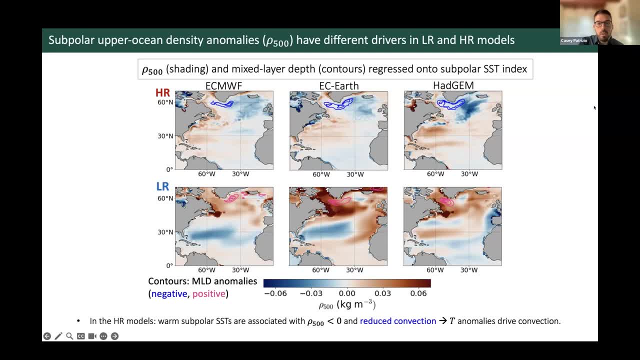 density anomalies tend to be associated with a warm subpolar SST. So if we focus on the HR simulations first in the top row, you'll see that warm subpolar SSTs tend to be associated with negative density anomalies in the subpolar region, as well as reduced convection in the western part. 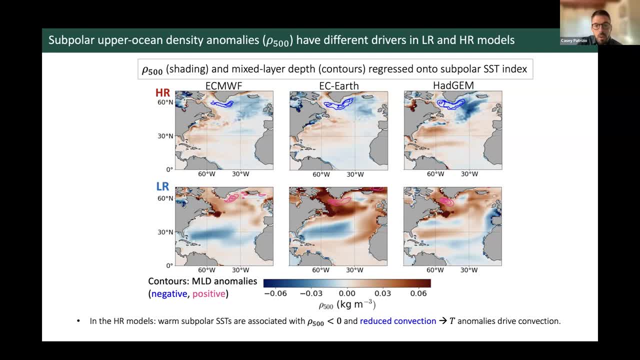 So this is the so-called Labrador-Eminger Cs. So, since we know that warming reduces density, this scenario is suggesting that the SSTs anomalies in the subpolar region are driving the convection that we're seeing. However, if we now move to the LR models, you can see basically the opposite scenario. 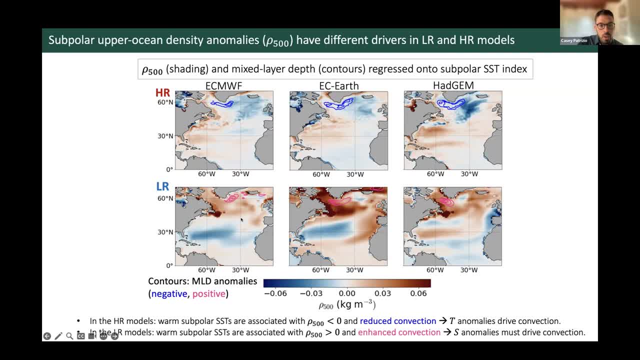 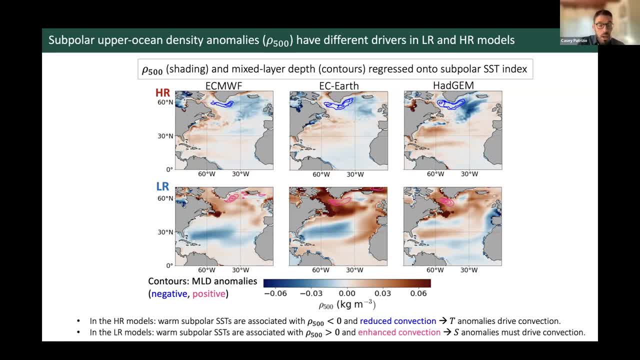 in this region to be driving the convection that we're seeing. So in this case, it's impossible for the SSTs in this region to be driving the convection, the enhanced convection that we're seeing here, And so this suggests that salinity anomalies are playing an important role in this region. 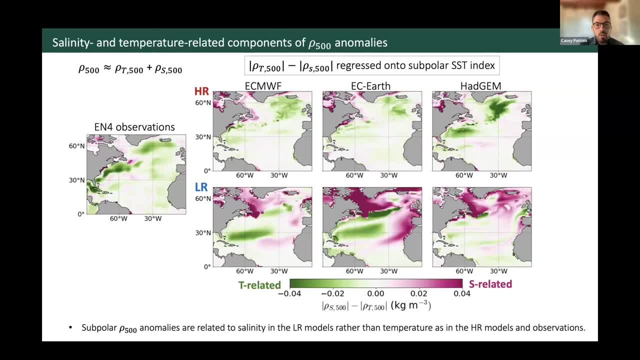 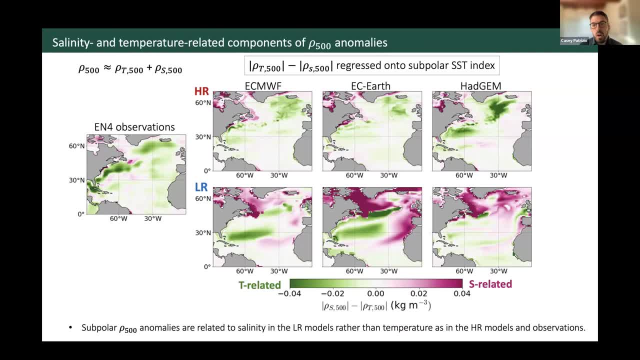 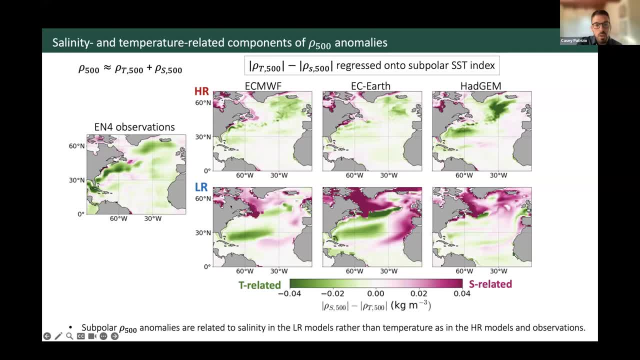 density anomalies, And this is clearly the case in the LR model runs. Interestingly and importantly, the HR simulations appear to be more realistic, at least compared to observations from EN4, which I'm showing here on the left. So this is quite an important discrepancy. 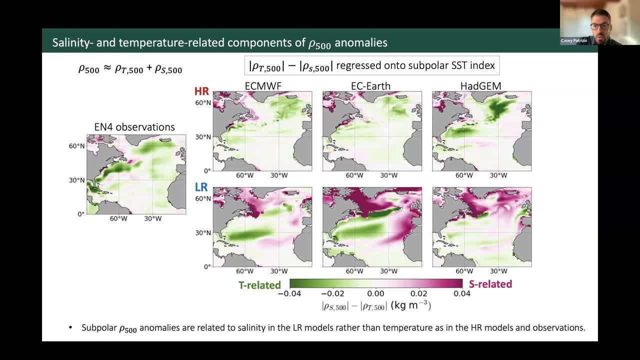 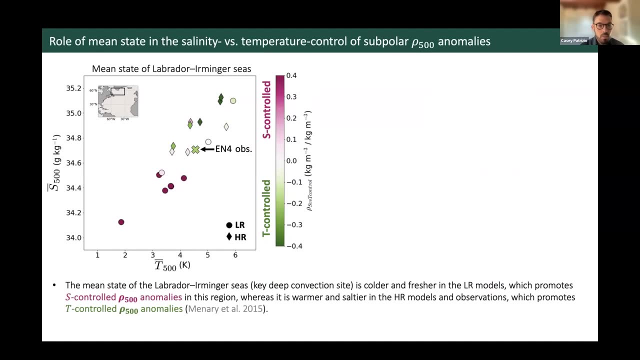 and ultimately it's going to explain the differences that we're seeing in ocean circulation variability. If you bear with me, I'll get to that in the end. Next, I want to just link the this to the mean state. This is ultimately what's going to explain the differences we're seeing. 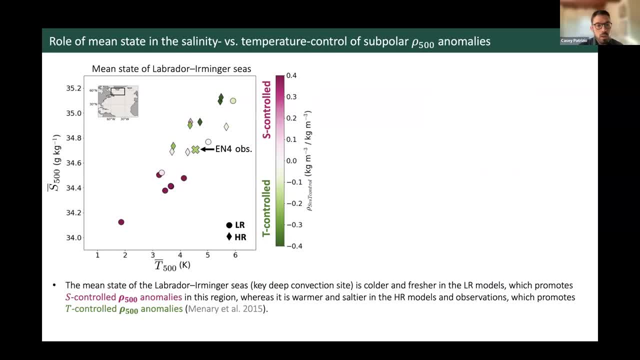 between salinity versus temperature-controlled density anomalies. So here I followed a method from Menry et al's 2015 paper and we calculated the salinity versus temperature-controlled density anomalies in the Labrador-Erminger seas. This is the key deep convection region that I identified. 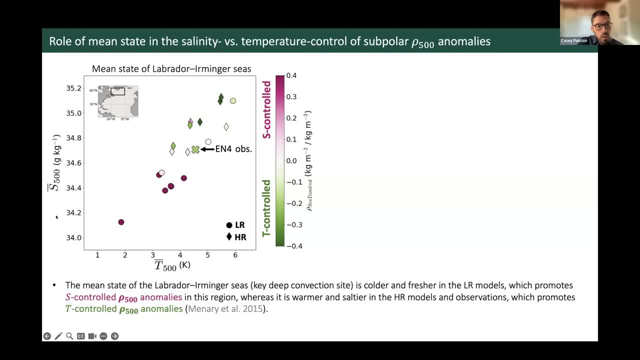 previously And we also calculated the upper-ocean mean salinity and mean temperature, And we've done this for each of the control runs in our study And so, as you can see, the LR models with salinity controlled density anomalies in this region tend to have a colder, fresher mean state. 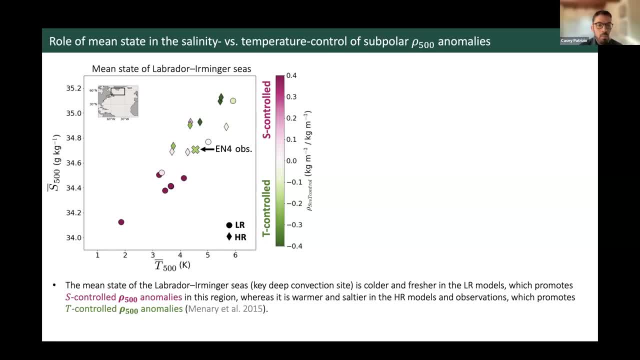 And this is in part due to having a weaker mean AMOC, as I discussed in the introduction. So, in contrast, the HR models- as well as observations from EN4, tend to have temperature-controlled density anomalies and a warmer, saltier mean state, And so Menry et al found a similar relationship in CMIP5 simulations. 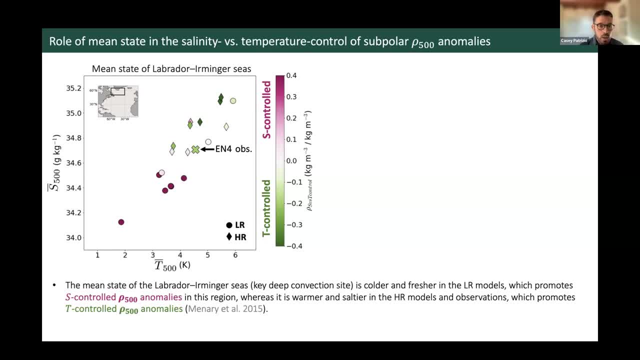 and ultimately argued that this is due to the non-linearity of the equation of state. So when the mean state is colder and fresher, this means that salinity anomalies tend to have a greater influence on density, And so it seems that similar arguments hold. 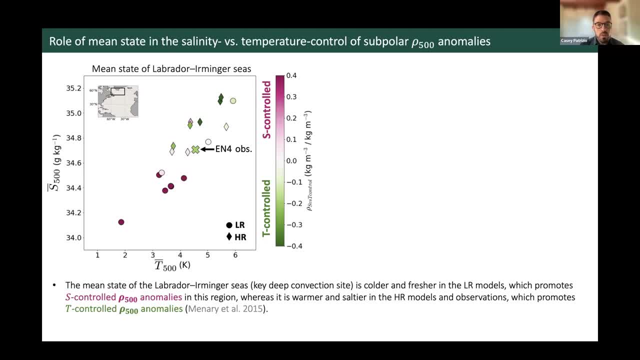 for the high-res player simulations that we've analyzed. Okay, So finally, coming to the variability, which is what we're interested in understanding. So in this plot, I'm showing the low-frequency variance of the resultation in n- curl- Rouge, which on average is less than 1,040bps, by the residual change in. n- Juan, which on average is less than 15,Yv of moisture, and it is all compared with a smaller reduction than earlier in the показыв lár del countries. 540달h died- 8,9,928aE. So these two are our safety variables. 9,088vs are characterized. The water thermometer generators give an. 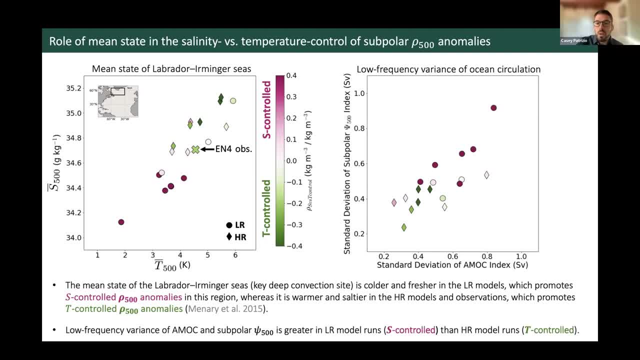 the low frequency variance of two different ocean circulation indices. So on the horizontal axis of the AMOC index and on the vertical axis of the horizontal stream function, averaged over the subpolar region. So you can see that the LR model runs with salinity controlled density. 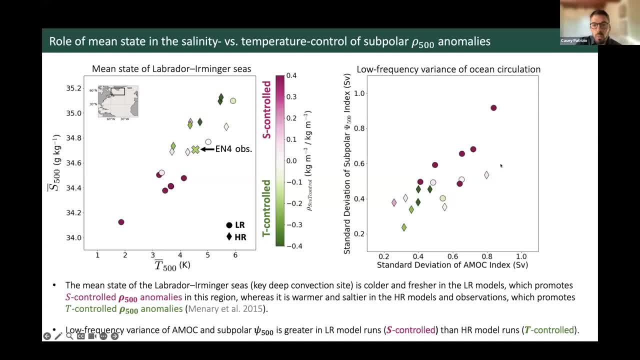 anomalies have greater variance in both of these ocean circulation indices as compared to the HR model runs, And so this link between cold fresh mean state associated with salinity controlled density anomalies is really quite well understood from previous studies. But why is this also associated with larger variance in the AMOC and subpolar variables? 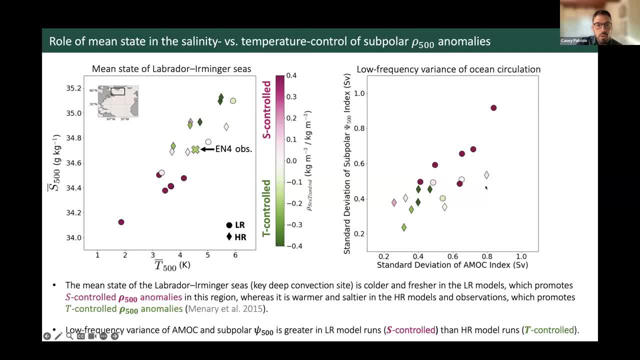 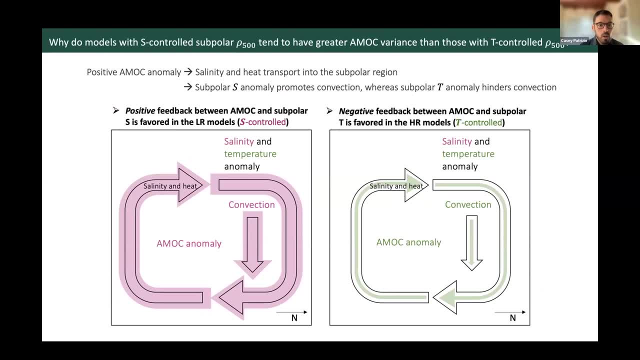 This is really the key to understanding our results. So the explanation we came up with is really quite simple. You can consider a positive AMOC anomaly which transports both salinity and heat into the subpolar region, So in this case, the subpolar 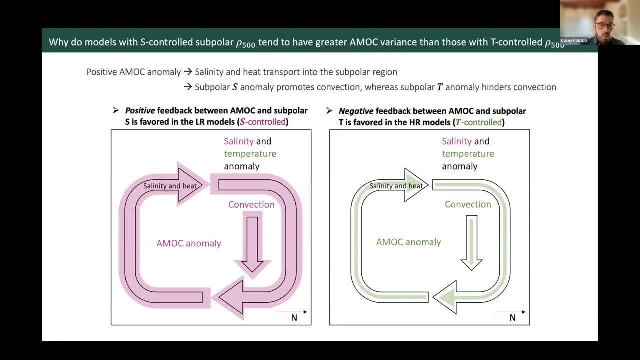 salinity anomaly will eventually promote convection and therefore act as a positive feedback on the AMOC anomaly. So this is really quite simple. You can consider a positive AMOC anomaly which transports both salinity and heat into the subpolar region. So this is really quite simple. You can consider a. 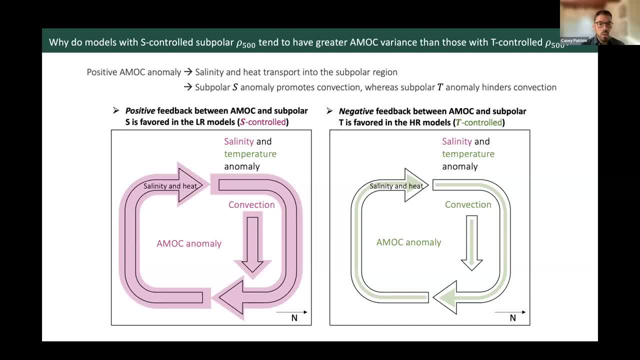 aresal initial AMOC anomaly as well as the subpolar variables, So this enhances low frequency variance. On the other hand, the temperature anomaly will act to hinder convection, acting as a negative feedback on the AMOC, And so, for these reasons, we're hypothesizing that this positive 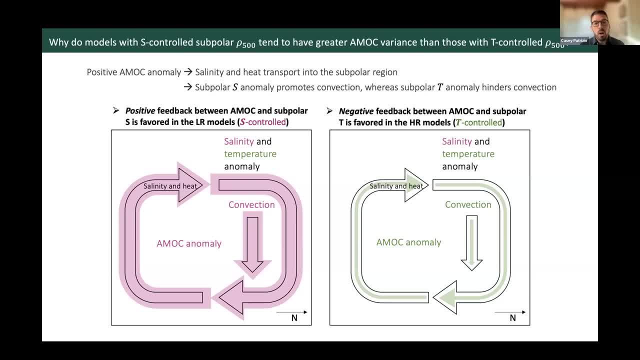 AMOC salinity feedback is favored in the LR model runs, And so this is really quite simple. You can Datte a basic take to a happening with a discrete prism were there'll be a positive salinity, subpolar けど, And so, for these reasons, we're hypothesizing that this positive AMOC salinity feedback is favored in the 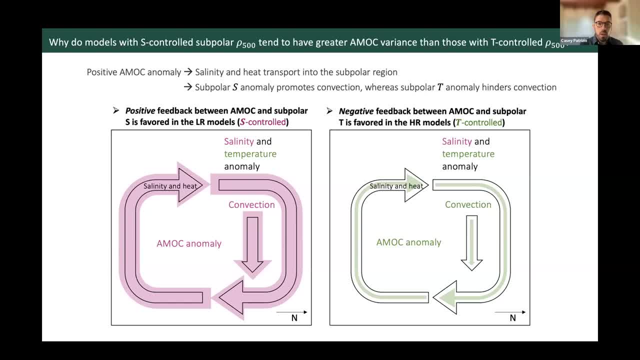 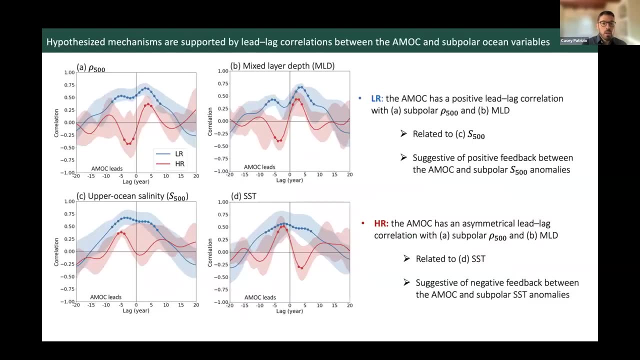 are more salinity controlled, whereas this negative temperature AMOC feedback will be favored in the HR model runs that are more temperature controlled. Just checking my time, Okay, So it seems that these mechanisms are supported, So here supported by lead-lag. 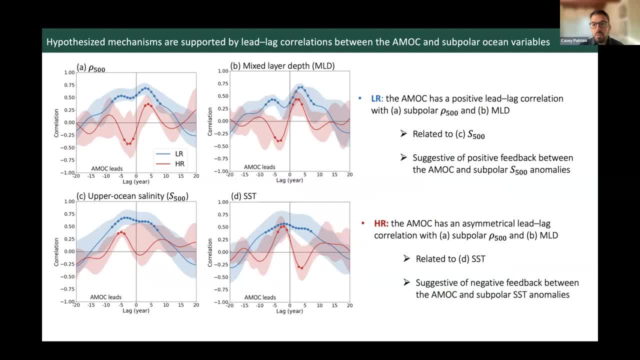 correlations between the AMOC and different variables averaged over the subpolar region. So in particular the LR model runs. the AMOC shows a much a positive lead-lag correlation with subpolar density and mixed layer depths, as shown in the top row here. 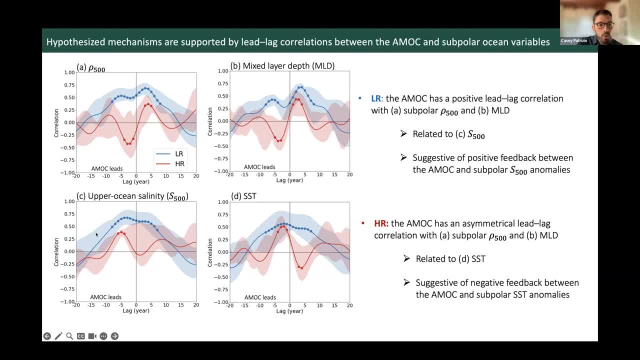 And this appears to be largely related to upper ocean salinity, shown in panel C here, as opposed to SSTs as shown in panel D. This is because the SSTs- the warming that we're seeing- would actually drive negative density anomalies. So it must. 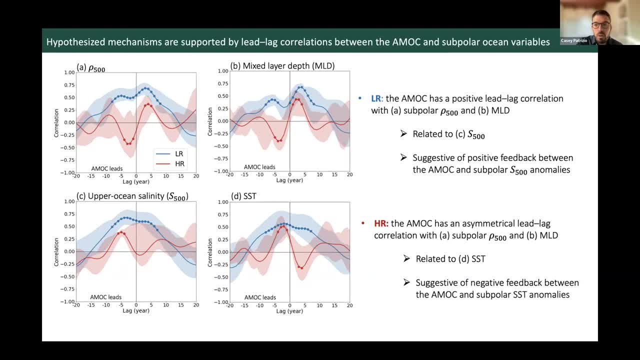 be related to salinity And this is suggestive of a positive feedback between AMOC and salinity anomalies. On the other hand, in the HR models we see that the AMOC has a much more asymmetrical lead-lag correlation with upper ocean density anomalies and mixed layer depths, And in this case, 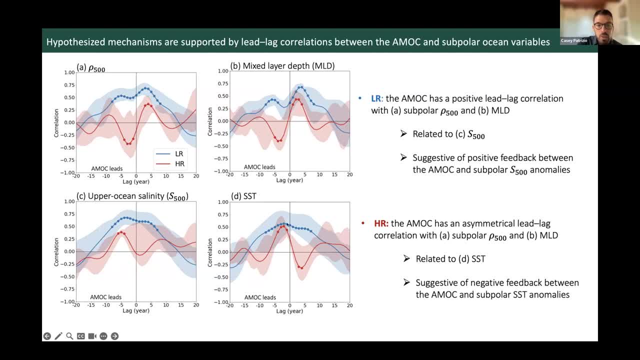 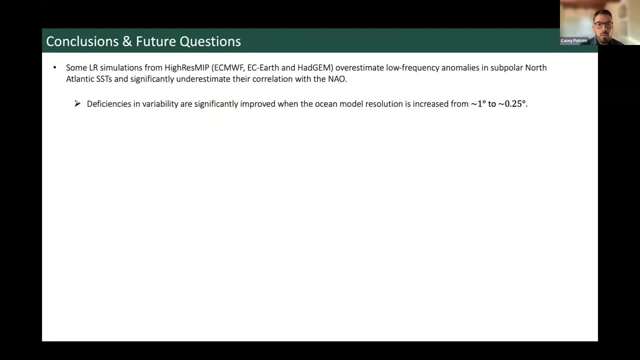 the correlation structure is related to SSTs shown in panel D and not salinity, And so this is also suggestive of a negative feedback between AMOC and subpolar SST anomalies. Okay, so, coming to the end, now I just want to summarize the findings and then discuss some 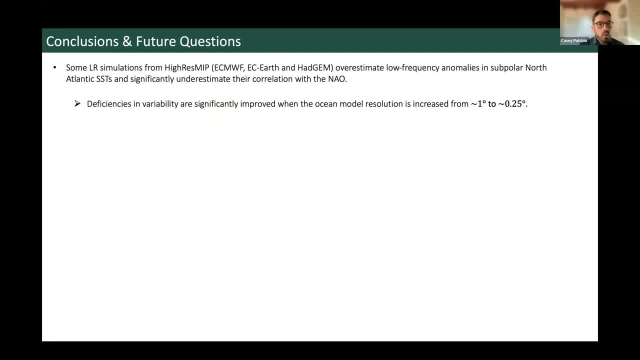 possible future questions. So we found that some of the LR simulations from the HI-RES MIP, notably ECMWF, EC-Earth and HadGem, overestimate low frequency SST anomalies in the subpolar North Atlantic region and then suggest that the AMOC as shown in the panel D is. 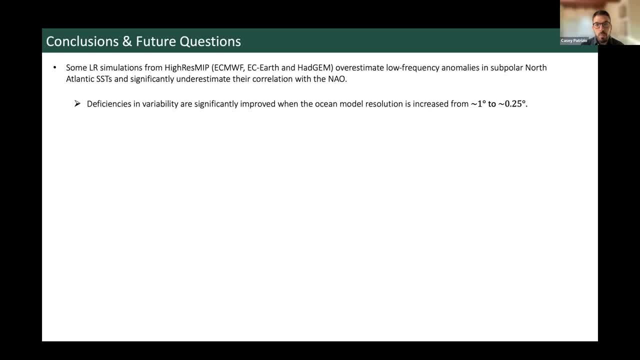 significantly underestimate their correlation with the NAO. We've importantly found that these deficiencies are really improved when the ocean model resolution is increased, and this is ultimately due to variability of the ocean circulation. So we found that the LR models have much greater low-frequency variance of the AMOC. 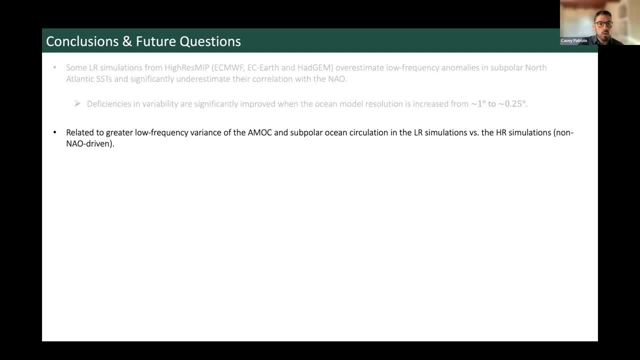 and the subpolar ocean circulation compared to the HR simulations. Ultimately we explain this in terms of differences in the upper ocean mean state of a key deconvection region which then promotes different drivers of AMOC variability. So the LR simulations have a colder, fresher mean state. 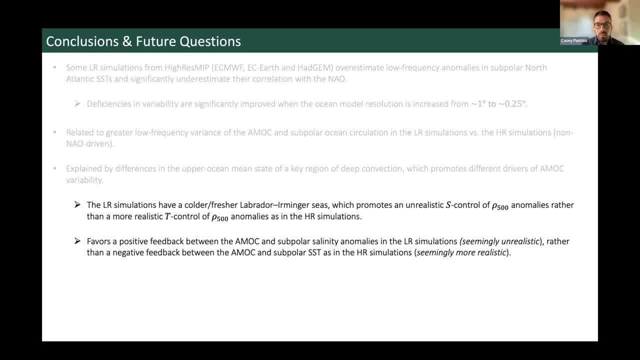 which promotes an unrealistic salinity control of density anomalies, leading to a positive AMOC salinity feedback rather than a negative AMOC temperature feedback that we see in the HR simulations, And so, lacking sufficient observations of the ocean circulation, we can't really form definitive conclusions about the realism of these different AMOC mechanisms. 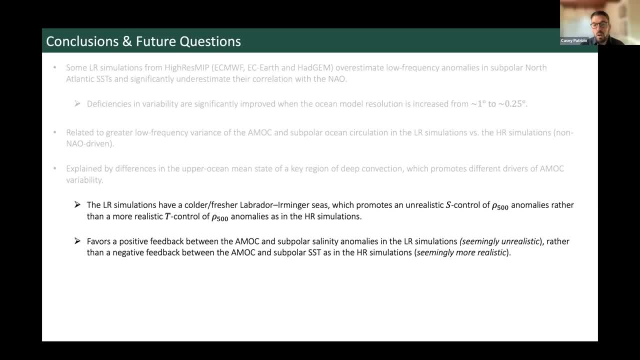 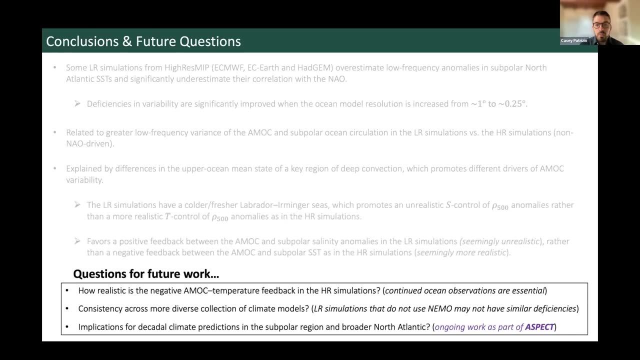 But it does seem that the HR simulations are more realistic, considering the results overall and considering the observational comparisons that we have made. In any case, I think this really does emphasize the need for continued ocean observations, particularly variables related to the ocean circulation. 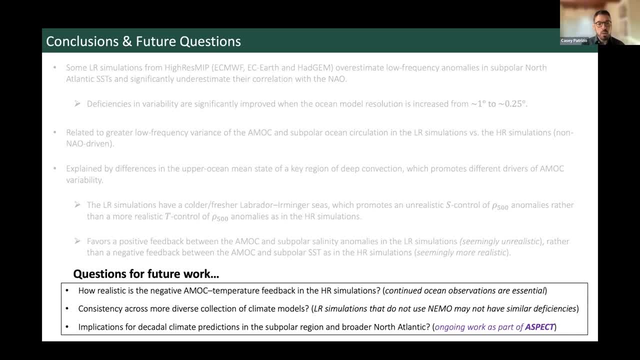 I also think it's important to consider the potential model dependency of these results in future work, And so I didn't have time to discuss this, but some of the LR simulations that we analyzed that don't use NEEMO don't appear to have any LR simulations. 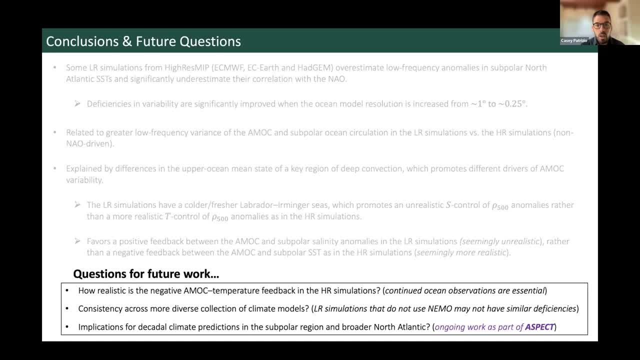 Some of them have similar deficiencies that I highlighted here and in fact seem to behave a bit more like the HR simulations, with more realistic SST variability. So for more details on that, you're welcome to check out the paper. Finally, we're interested in exploring the implications of these results for decadal climate predictions. 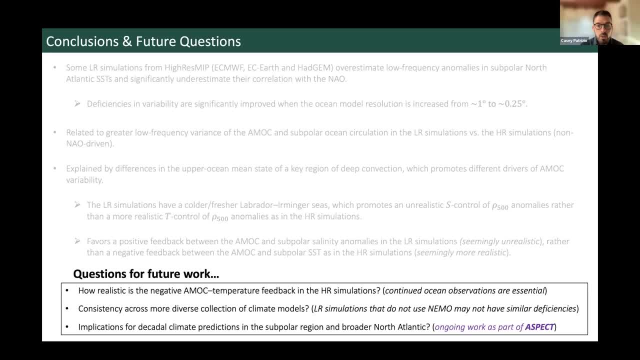 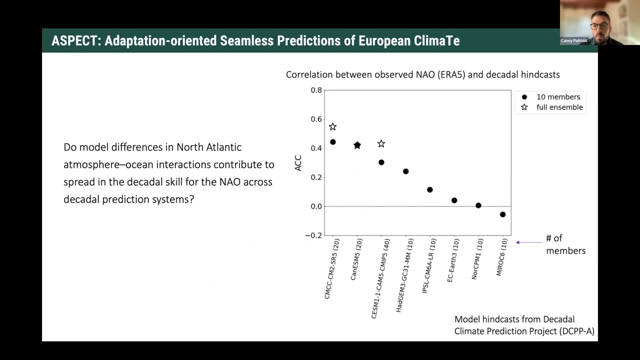 And so this is actually ongoing work as a part of the EU Horizon project aspect, And so, since I have probably a minute or two left here, I thought I'd highlight some of the ongoing work that we're doing as a part of aspect. And so, if you mentioned all the way to the beginning in the introduction, 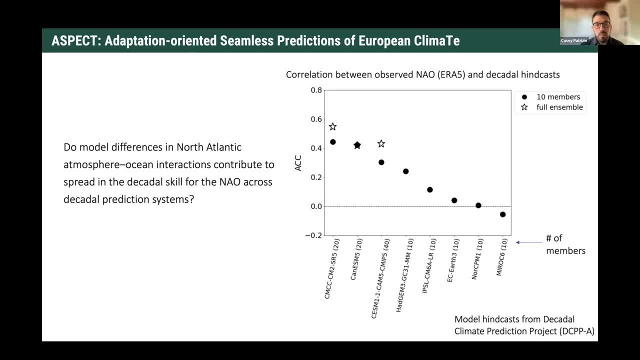 I mentioned that some studies have shown that the NAO may be predictable on decadal time scales, And this is something we're really interested in Here. it seems to see an understanding better And in particular, I've been focusing on understanding the role of atmosphere-ocean interactions in the North Atlantic. 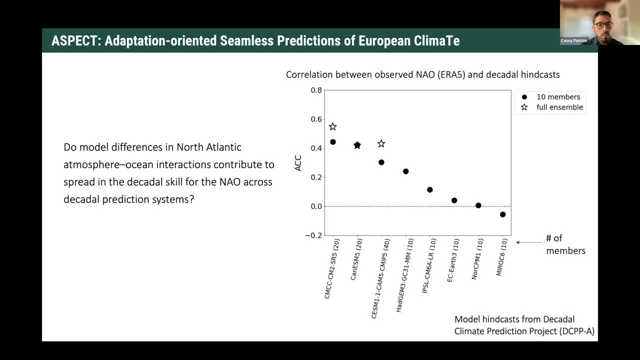 in decadal predictability of the NAO and whether model deficiencies contribute to spread in decadal scale for the NAO across different decadal prediction systems, as shown in this plot here on the right. So there I'm showing the correlation between the observed NAO and different decadal hindcasts from the decadal climate prediction project. 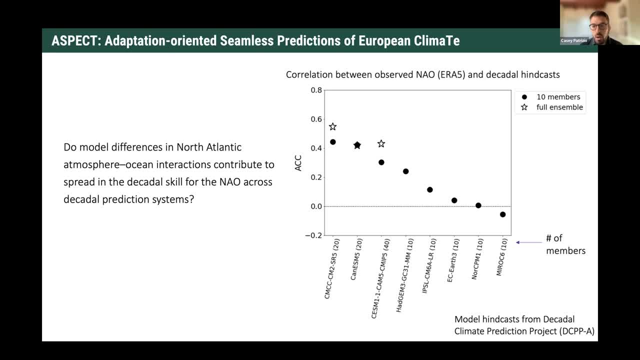 And so you can see that some models do a lot better than other models, And we're interested in understanding whether this is linked to deficiencies in North Atlantic atmosphere-ocean interactions. So yeah, hopefully we'll have interesting results on this in the future. 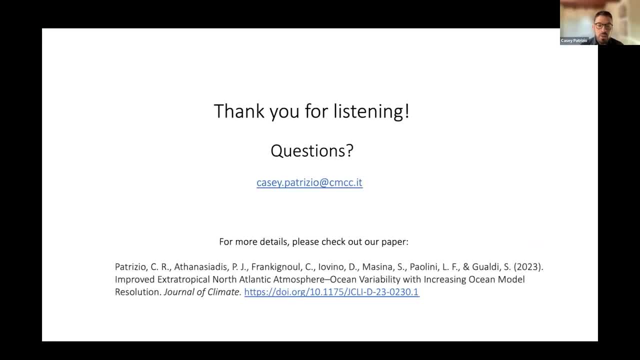 Stay tuned for that. For now, I'll just thank you for listening and thanks for joining this webinar. I'd be happy to answer any questions. Let's see Excellent, Casey. Thank you very much Again. I would like to apologize to everyone for losing my connection at the beginning. 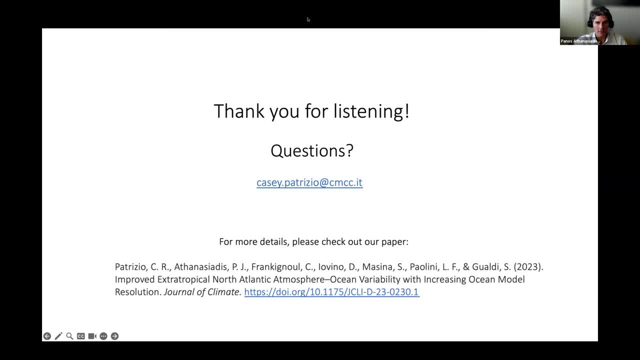 We welcome questions. Also, feel free to raise your hand in the question and answers section. There is already Franco Boscolo who would like to raise a question. I suppose, Franco, I don't see your question. You haven't typed it fully. 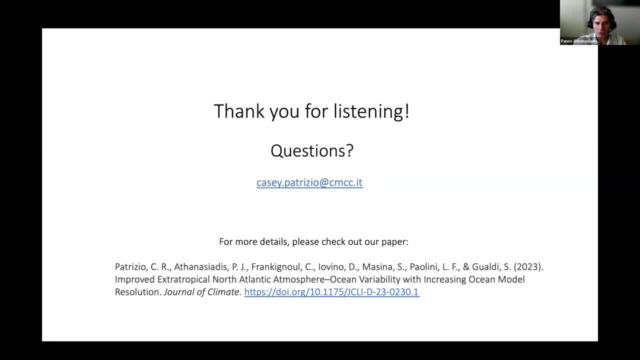 So would you like to raise your hand, Speak out. If not, there are other questions also appearing, So there's a question from Justin Mwangi And I'm reading it out from the question. from the asset is typed: Can high-res MIP be used to investigate? 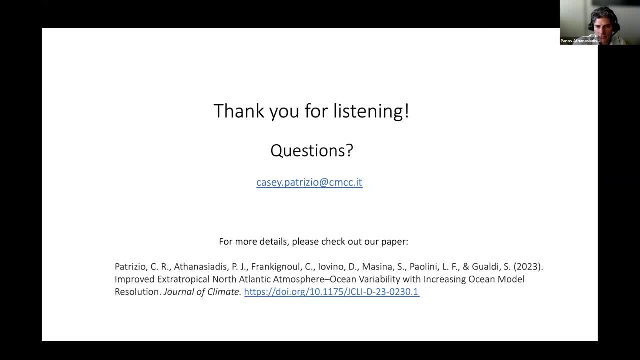 To investigate atmospheric ocean responses to deforestation, afforestation, reforestation. This is one question for you, Casey, Interesting. Should I read it again? No, I heard it. Yeah, there are lots of different applications for high-res MIP. 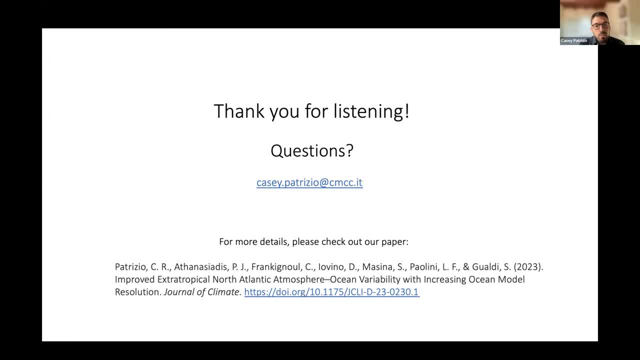 And I think I'm excited to see more work coming out of it. With regards to afforestation, deforestation, I'm not exactly sure that we could isolate that specific part, But it's an interesting idea And, yeah, I'd be excited to see, like I said, all kinds of creative work coming out of high-res MIP. 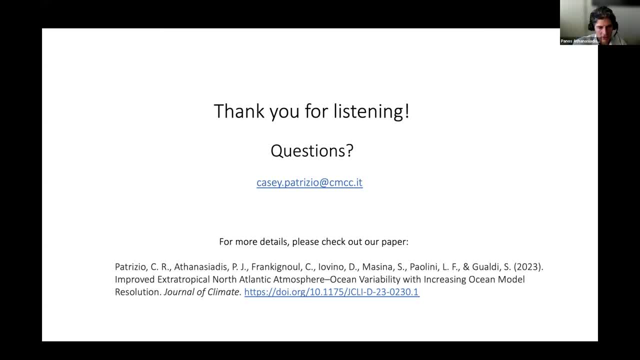 This is indeed a little bit far from what you presented here, But yes, let me also mention there is a question coming in from Malcolm Roberts from UK Met Office. Malcolm, I'm reading this for you, since you type it down: Do you find similar excessive long timescale variability in C-MIP models? 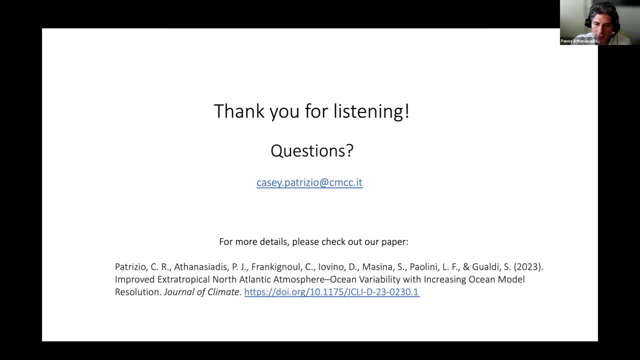 I mean these high-res MIP simulations contributed to C-MIP. So there are always questions in high-res MIP about spin-up, ocean adjustment etc. Any comments? Casey, Yes, it's a good question. So I personally have not analyzed all of the C-MIP simulations. 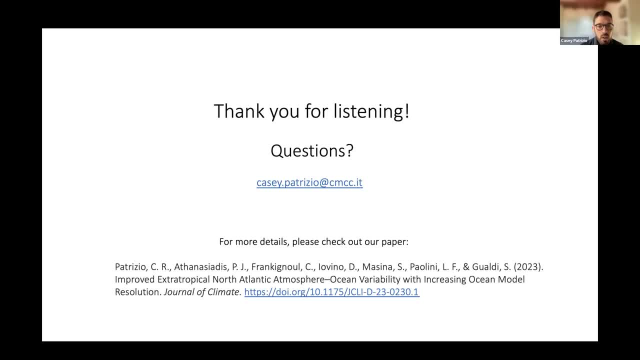 But there have been some studies that have shown have looked at this in more detail And there does seem to be actually more models that may underestimate low-frequency variance, And so it's possible that there is a model dependency of results here. I think still it would be interesting to look at dependency on mean state across the C-MIP models. 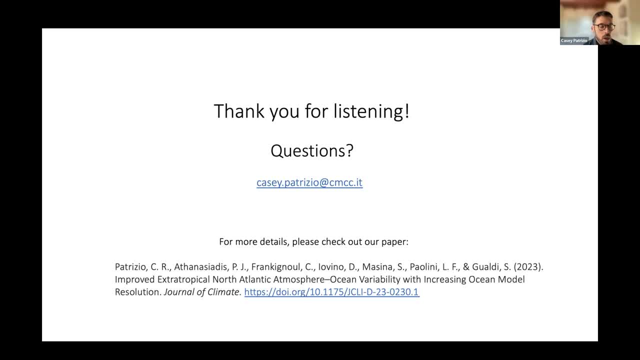 And whether those models that have underestimated low-frequency variance maybe the mean state is actually not colder, fresher, like we showed in the LR simulations in high-res MIP. So yeah, in terms of spin-up, I think yeah, that's a potential concern. 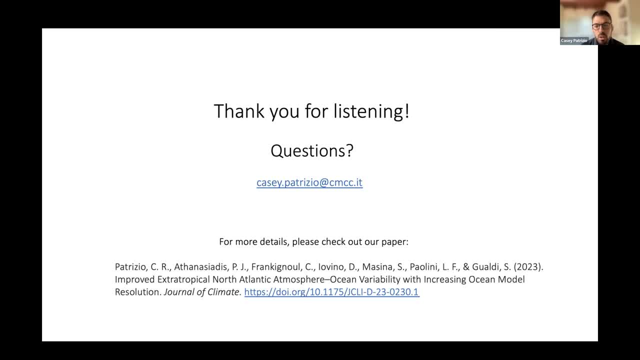 I think in the high-res MIP simulations, if I understood, they are run for a certain period of time before the control of C-MIP And before the control runs and before the historical runs to try and deal with the issue of spin-up. 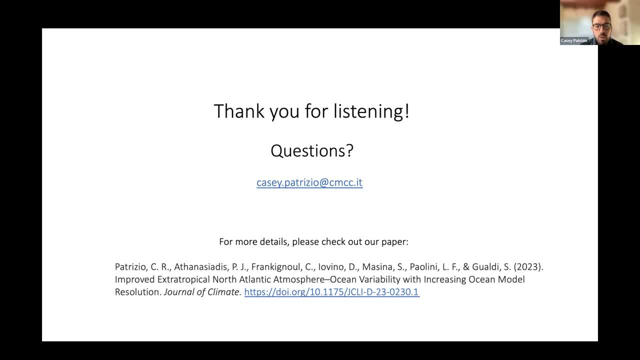 So hopefully that's not impacting the results too much. Yes, that's right, There is- Malcolm knows better. there has been a spin-up. I'm saying for other people at least 30 or 50 years, at least for high-res MIP. 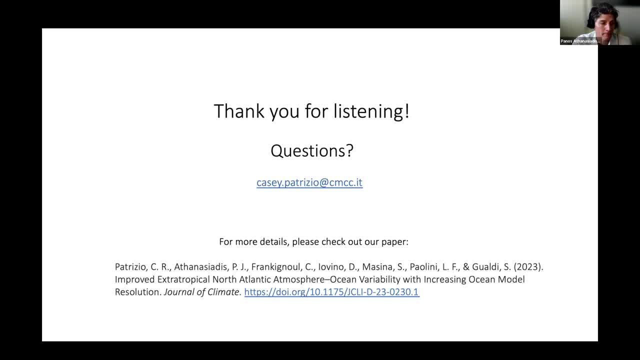 Hmm, Of course, as you mentioned, Kezi, I mean these models that you analyzed here, you presented, are mostly NEMO, And at least your work indicates that this provides an example of increasing model resolution. Ocean resolution is not a remedy for all models, for our systems. 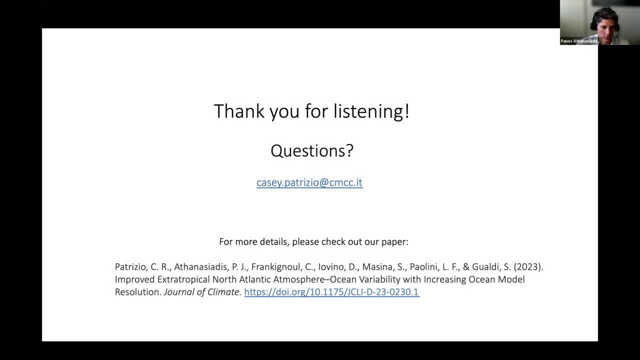 Yeah, But at least here we can see that And what consequences we may have in a modeling system when resolution-related issues play a role, as you demonstrated. There is another question and we still have five minutes to go, So let me raise this from the chat. 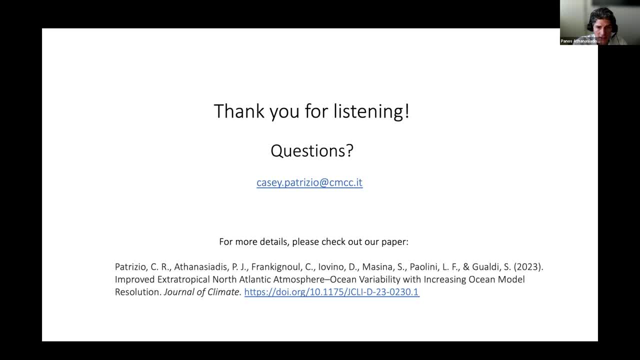 Chris Danick asks. thanks for your presentation comments. So in frequency space low-resolution models have more variability, As far as I know, in wave number space the situation is reversed. Can you speculate on that? Thank you, And yeah, sorry, I have no microphone available. 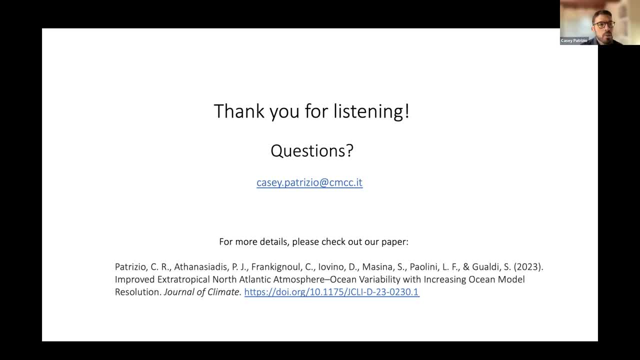 Okay, No worries, Yeah, that's an interesting point. So I understood. So in wave number space, yes, the high-resolution simulations will have more variance on smaller scales in general. And in frequency space, we're seeing the low-res models have greater variance on low-frequency timescales. 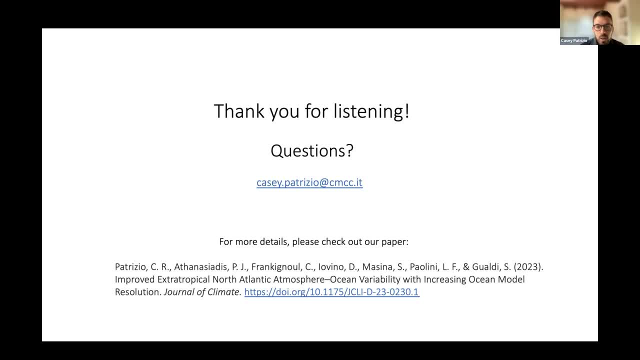 So this is something I thought about before At the beginning of this, And whether there's a relationship between these two things, But I couldn't personally come up with a good explanation And I think perhaps it may just be a coincidence- I wouldn't necessarily expand this to anything more than a coincidence. 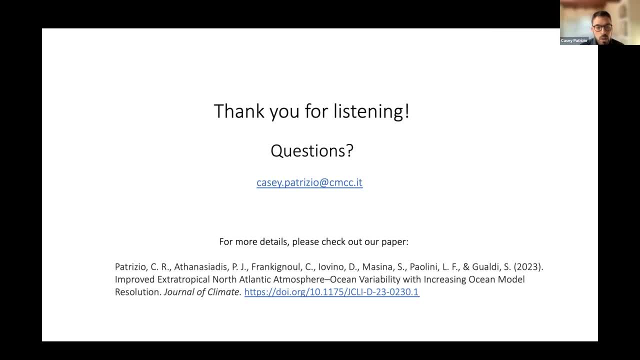 Particularly in this region. It seems to be more related to mean state as opposed to the other two. I don't think so. Yeah, I think it's more related to something more fundamental going on. So yeah, I'm sure I didn't answer your question directly. 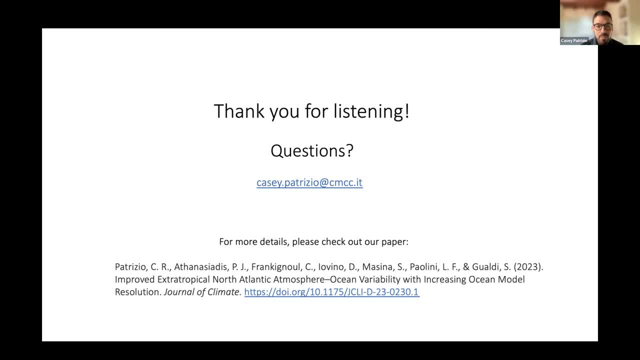 But that's the best answer I could give. Thank you, Kiersey. One more question, I see. Since there is no raised hand, I will continue reading the questions from the session asking kj uh hi. thank you for the interesting presentation. have you considered other boxes? 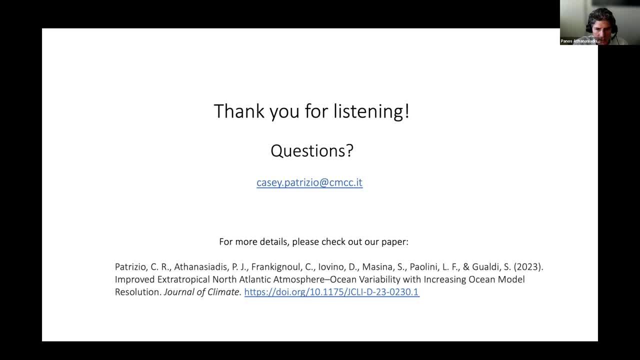 for your regression analysis. in parentheses figure about upper ocean density: density at 500. anomalies regressed onto the standardized subpolar ssd index. so have you considered other boxes? and it was found that different models might have different deep convection regions depending on resolution. yes, so the first question. we have played a little bit around with boxes, a little bit so for the sst. 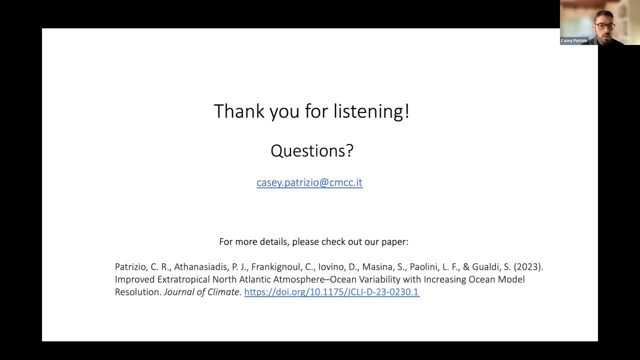 indices, the boxes didn't really matter too much. so we could, you know, expand that, decrease that and the results are fairly similar. referring more to the uh, labrador, emminger seas, uh, so the, the, the salinity versus temperature control. in that region there's some sensitivity. 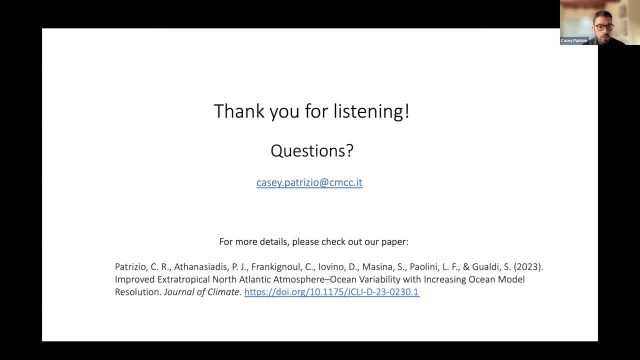 to the box that we choose there. so if we, if we focus more on the labrador seas, we see more salinity controlled density anomalies. if we expand the box to the to the eastern part, so into the air minger seas, we get more temperature controlled density anomalies. 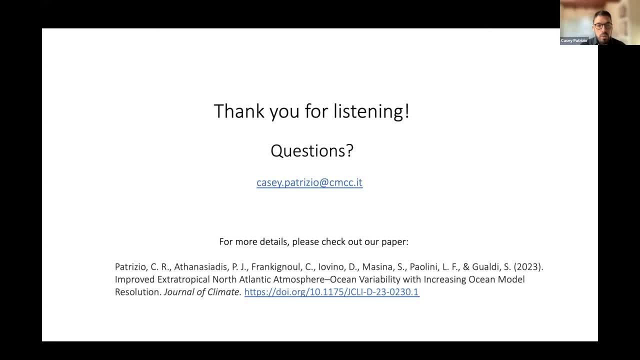 so some dependency there. in terms of the second question about having deep, different deep convection sites, yes, uh, it seems that uh hr models have more of the convection in the labrador seas in the western part. the lr models exhibit a little bit more convection, uh, in the eastern. 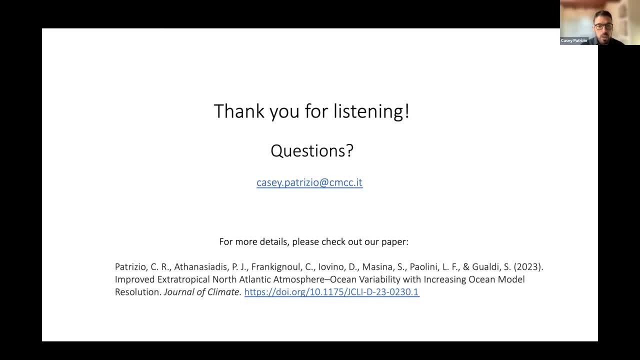 part. uh, in terms of variability, though, it seems that both lr and atri models exhibit variability in this labrador emminger seas that seem to be common to both of those models, uh, at least with respect to sep, polar sst variability, and so that's the reason why we chose that box centered on that region.